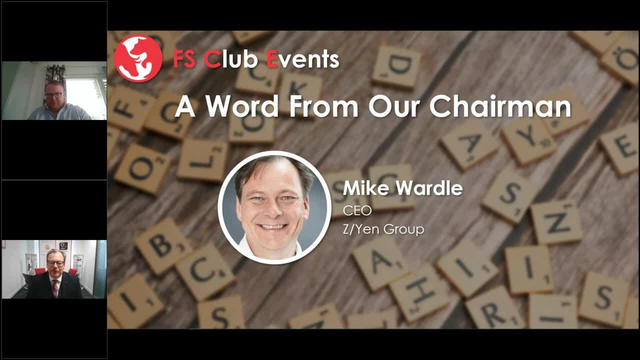 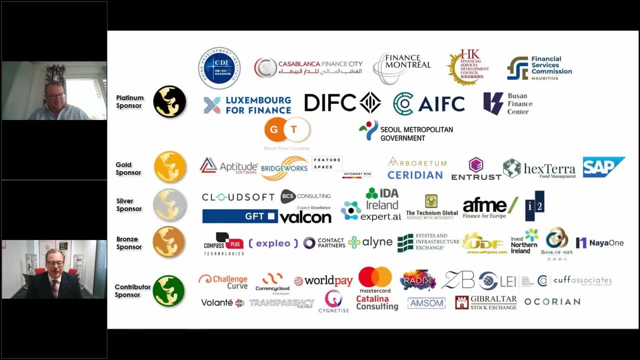 the questions towards the end, And the first thing to say is a big thank you to our sponsors. We're very lucky at CEN and the EFS club to have a range of sponsors who enable us, through their generous support, to run this webinar series and other events and to range quite widely over the 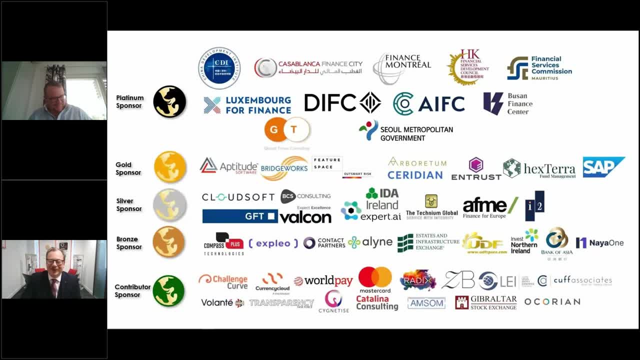 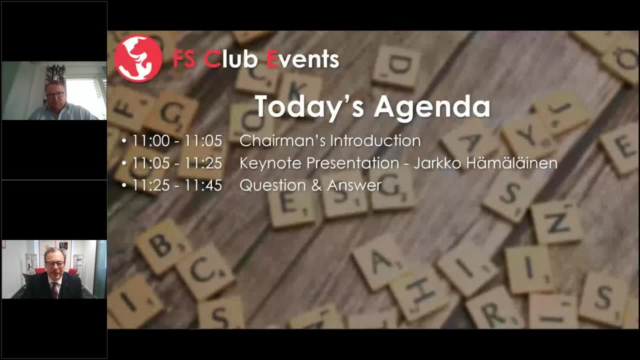 questions of economics, finance, science, history, you name it. The programme today is fairly simple: very short introduction from me and then we'll have around about a 20-minute presentation from Jarkko As our keynote, and then there'll be time for Q&A towards the end. If you haven't used the GoTo, 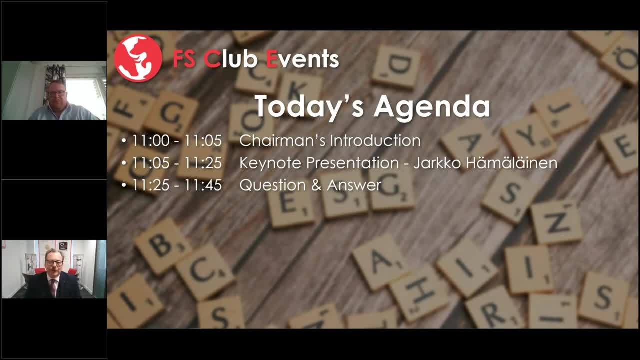 webinar system. before the way to put in a question or a comment is to find the question tab on the dashboard on screen type in your question and that will come to us to feel during the Q&A session. And please do put your comments and questions in at any point during the. 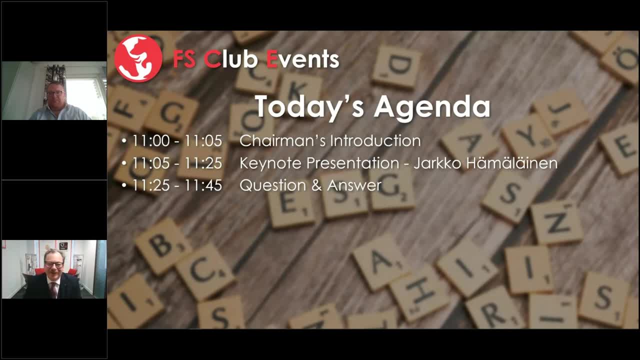 presentation. If you have a good idea or thought, get it down so that we don't miss it. And just to say that we will share contact details with those of you who ask questions with Jarkko, so if there's a need for any follow-up discussion, that can be made easier. 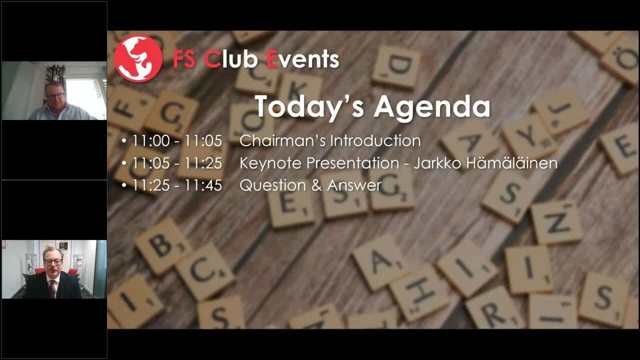 The session is being recorded today, and so if you want to go back and refresh yourself as to Jarkko's presentation, or you want to share the session with friends and colleagues who might be interested, the link to the recording will be up on our website in about 24 hours and that'll be available for you. 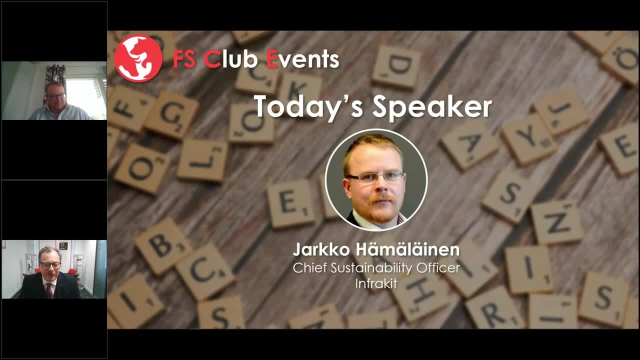 to share. So that's all, I think, by way of housekeeping and introduction. It's a great pleasure to introduce Jarkko Hamerleinen, with a more than 20 years global background, including with Nokia, Hewlett-Packard and the CEO of Startups and consulting with many very large 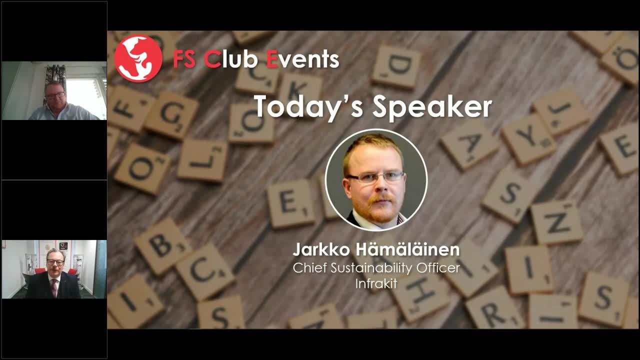 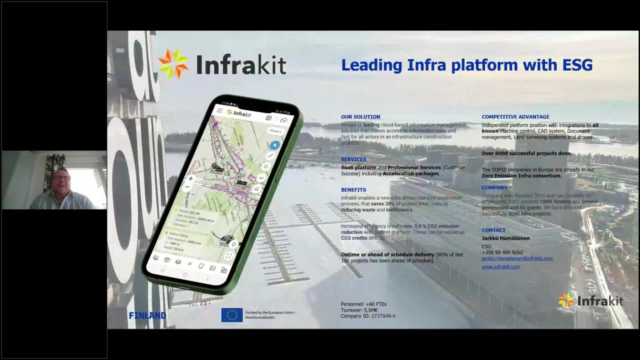 companies And really looking forward, Jarkko, to what I know has been a long progress of development in your thinking around ESG, and really looking forward to your presentation Over to you. thank you, Thank you, Mike. So it's a privilege to be here and I need to share a little bit my story. 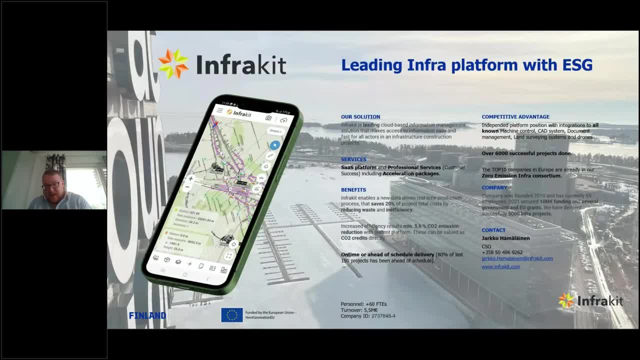 because my dad is actually the construction guru and he has close to 60 years experience from construction and once we were sharing or even comparing kind of my experiences from Nokia, Amazon, General Electric, Hewlett-Packard and many of the construction of companies like a canary wolf, british land- uh, wanda and mr, just to name a view- and i was asking: 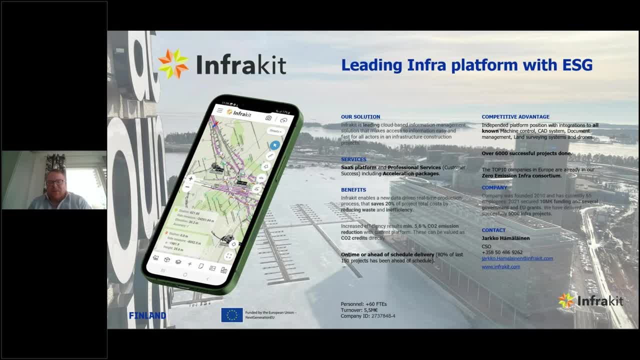 my dad like what has been the biggest innovation, uh, during your career? and that time he was still smoking a cigarette and he was taking taking a couple of kind of a breath and saying that my son, you, you remember how the toilet used to be like this and nowadays he's just pushing the button. 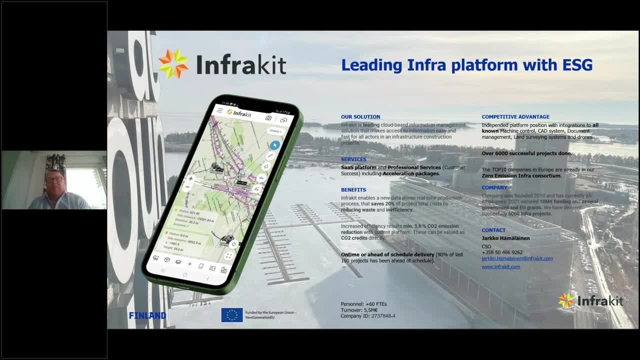 so that was a message. i of course a little bit was laughing, but taking it so seriously that one day i will give my kind of a best competence for the construction in a in a form of digitalization and esg. and very same story happened in the beginning of infrakit. then, uh, temu kivimaki ceo and founder. 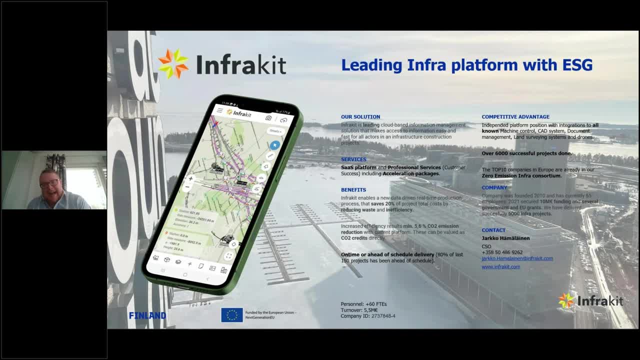 was looking for master thesis- and it was not his dad, but it was the professor from oulu, finland, like our local silicon valley, that why don't you focus to infra construction and enable, like digitalization and data moving uh to and from machines on site? and then that was done and the first customer it was 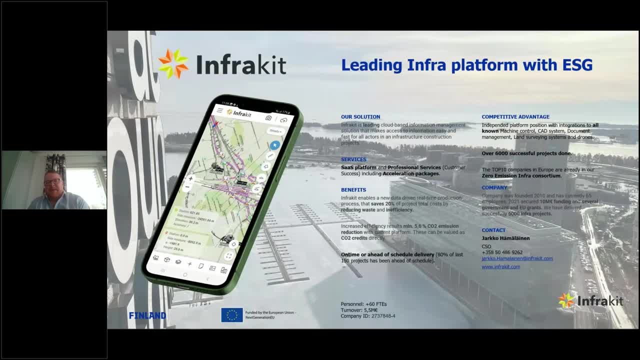 called testia, like a government-owned, like highways company in finland. so, um, they started digital like a journey 13 years ago and then they started to build a company. and they started to build a company called colas, and they got actually acquired two years ago by huge company called. 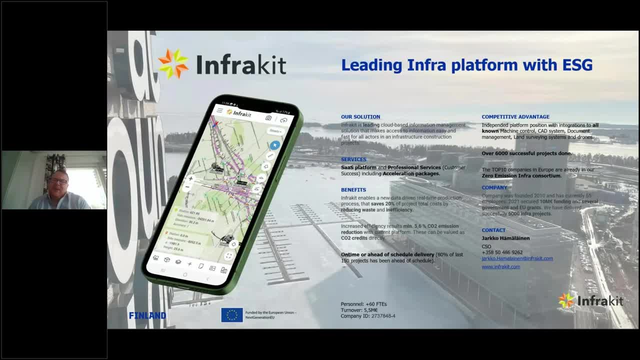 colas and then i joined. i wanted to understand what was the customer impact when we have been focusing to build digital and esg services. and uh, we went through like, uh, like pretty much talking directly to the customer key uh personnel and saying like before digitalization and esg and after, so how can 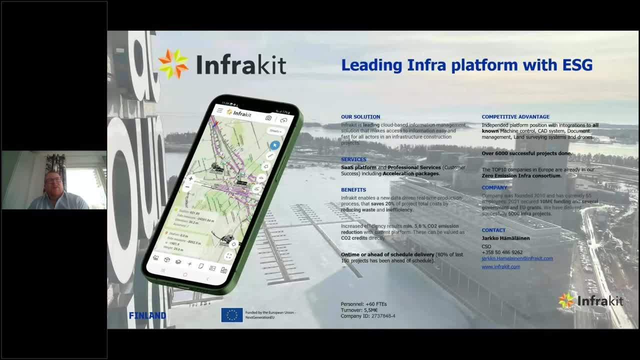 you see your change. and the first answer was: we win all the projects we want, we won't want. and uh, they, they actually won 10 out of 10 projects, all the big ones, all the meaningful ones. and then i said that, wow, that's like. uh, you became number one. what? what else happened? like like, have you find any other? like, 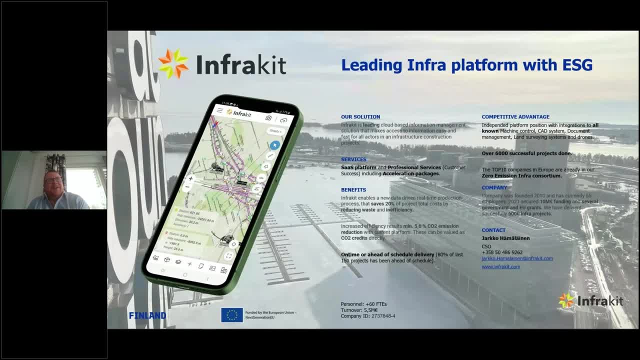 uh, when you are able to to solve your actual esgs. so what else happens? that you are winning the projects? and the answer from customer was: uh, we are able to make it 20 percent on the part of the customer. and the answer from customer was: uh, we are able to make it 20 percent on the part of the customer. 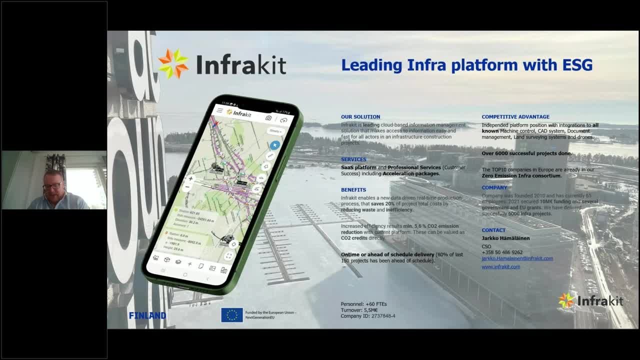 budget and i thought that 20 percent good or bad. so, being in a different industries and i had to google that- and infrastructure margins are between four to five percent, so yeah, it's pretty amazing. and then then after that i wanted to put all the effort that can we prove from esg point of view? 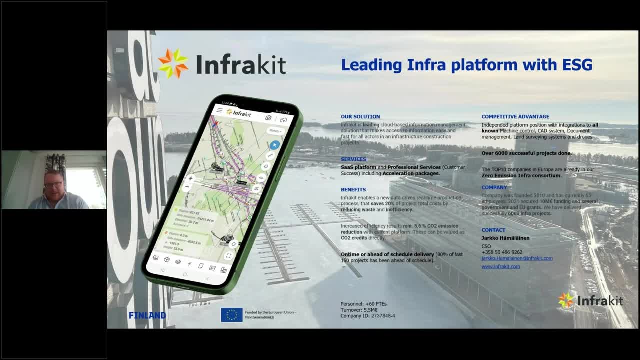 like what all environmental, social, governance, sustainable and co2 reduction impact we have if we, if we utilize digital platforms and uh and we can, we can have real-time esc actuals. so that was one of the biggest findings: that the outcome was very positive, in the worst case, without even demanding 5.6. 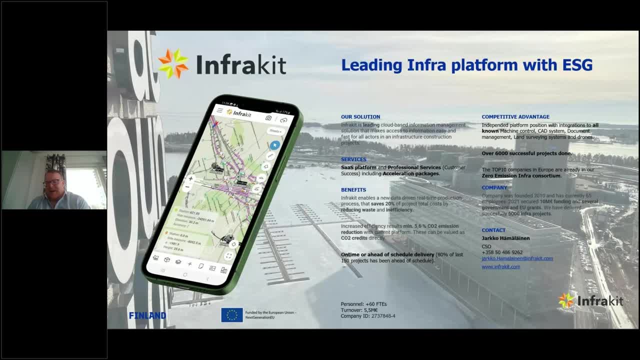 less co2 emissions. but how it was done it was get rid of waste, get rid of unnecessary movement, because when everything is digital, everybody knows what's happening when to do your part. so it's not a rocket science, it happens automatically. and then i first time realized that efficiency and sustainability can be hand in hand. and then then that story continued. 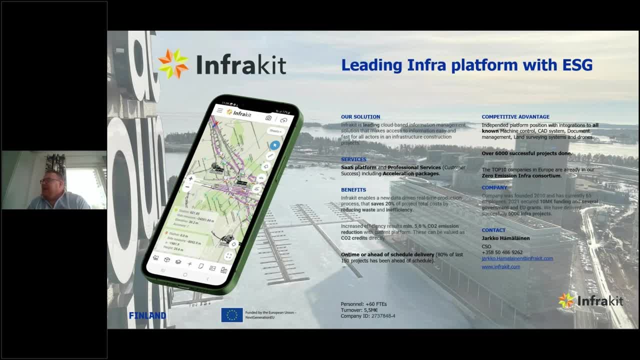 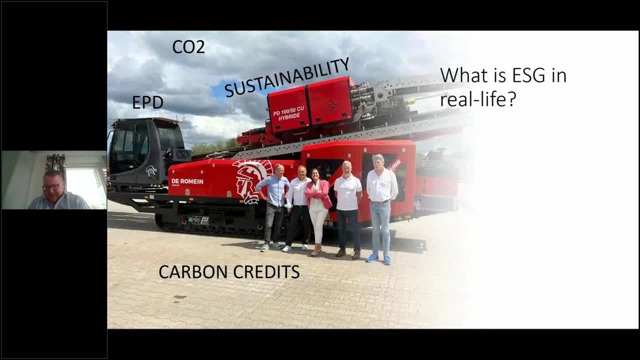 so if we can get the next like this. so after 6 000 projects. so we wanted to to kind of understand what else is esg than co2 reduction? uh, how, how should we take it from business? is it like a big advantage or is it some mandatory thing like uh, doing a kind of a corporate sustainability? 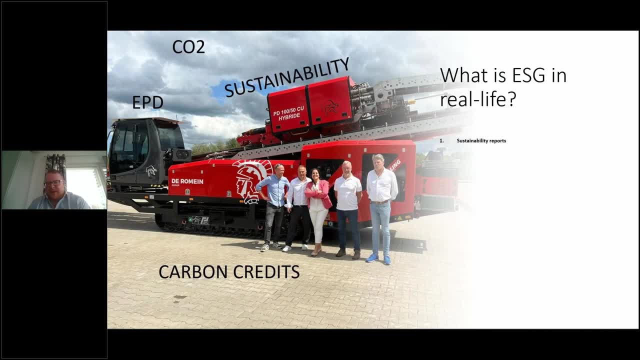 reports or is it just doing a sustainability report every year and look good? and then we continued asking, especially from owners like municipalities, cities, governments in europe, like uh, do you take esg seriously? and of course, from private owners and the main contractors. and and the first question i got, like do you take esg seriously? and there was executives from 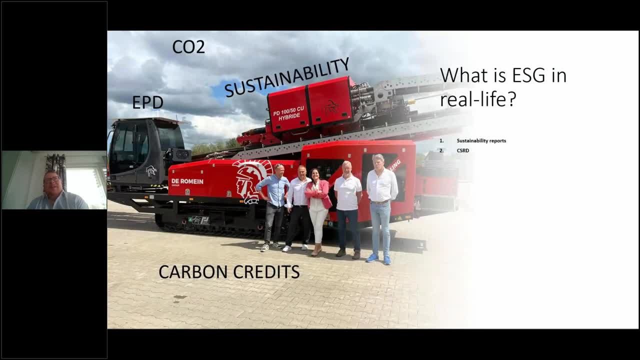 hilton, mr xavier walker was saying to me that jarko, money doesn't move if you cannot prove esg. and then i was. that was a couple of years ago. i liked the answer but couldn't understand it fully. nowadays i might understand it and of course i was asking explanations. 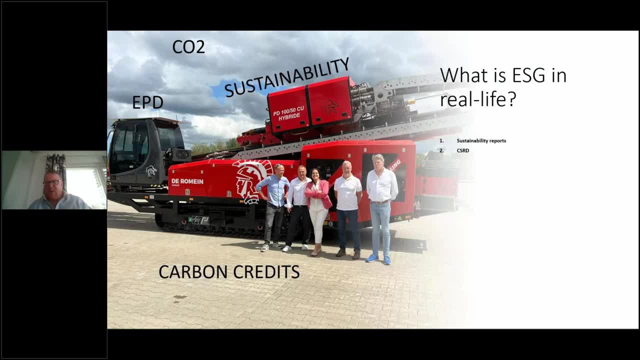 and and xavier was explaining that- as an owner, when you demand esg, so the the engineers and design guys and architects are involving esg criteria into plans and that goes to main contractor, subcontractor and you will be getting premium quality on time, so your asset value is higher. 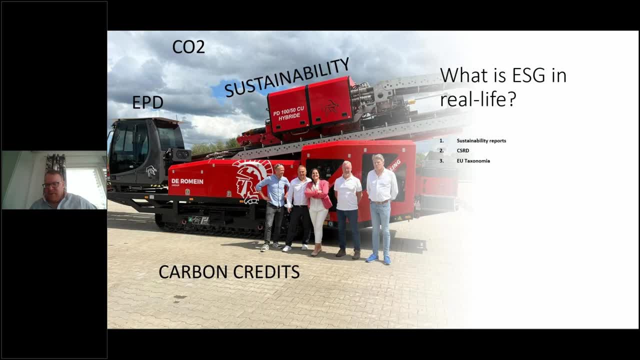 if you compare getting delayed. so it's not only more co2, it's also losing money and losing reputation. if you need to go all the way to fight about invoices or quality or whatever, so it actually begins like a court case and your asset value is slower. so that was huge and that's why i want to. 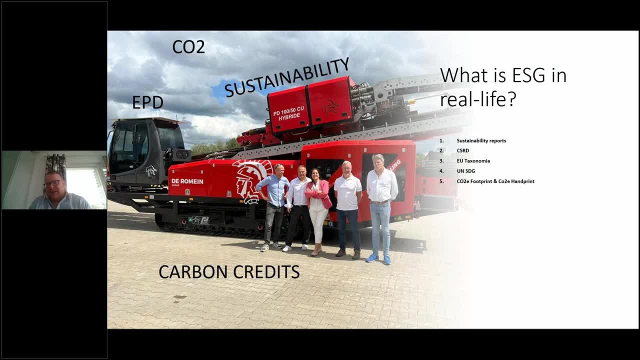 open our minds, like when we just look for esg, uh, from one angle, it's not enough. so, on top of your reports, there are deadlines, european union taxonomy- there is you and the kind of, uh, sustainable development goals- uh, there's, there's a lot of calculation: how much co2 equivalent footprint. 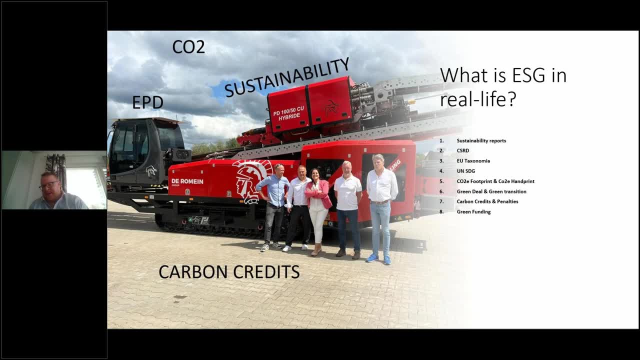 our companies have. how about the handprint via customers? how we are impacting huge green deal and hell of a lot of good money available. how to get it? there will be penalties. there will be carbon credits. there is much better funding available when we can fulfill the green funding. 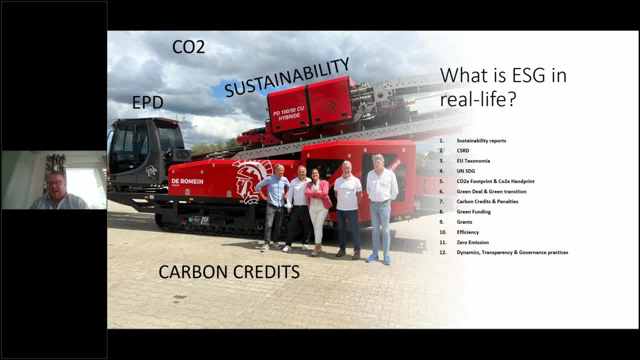 and green funds. there's really much european level and under country level grants for the kind of every kind of efficiency optimization using ai digitalization. there is uh like really much action with the best concert teams to zero emission, and there is, of course, all the dynamics, all the kind of uh transparent, uh kind of uh governing. 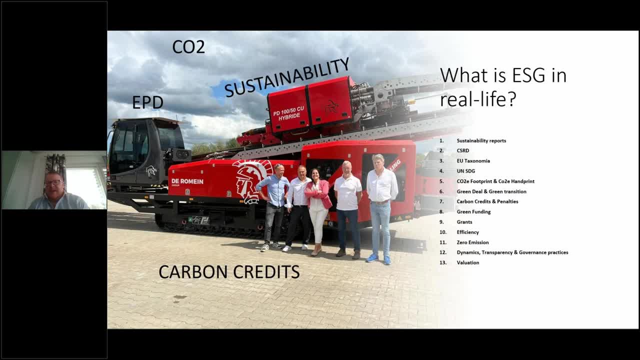 and i'm showing transparently all the good practices. and then there is valuation to your own company and to your own work and competitive advantage. so just an example: so so company i'm working for four years ago valuation was, uh, somewhere between four and five million euros. 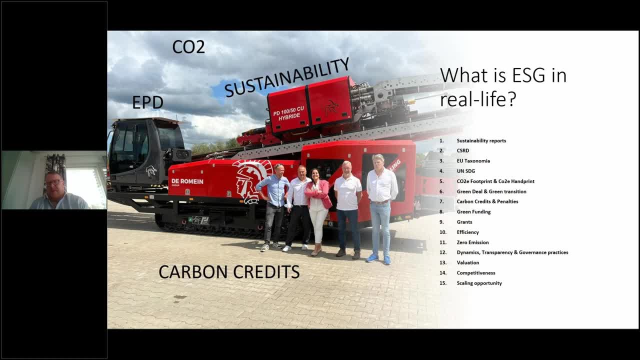 and uh. last spring it was closer to 200 million euros. so in a few years, uh platform, ecosystem, neutral platform for esg services and for infrastructure, valuation has been rising so rapidly. so how it's possible if we wouldn't have this esg trend- people demanding esg and then we are enabling it. so i would say 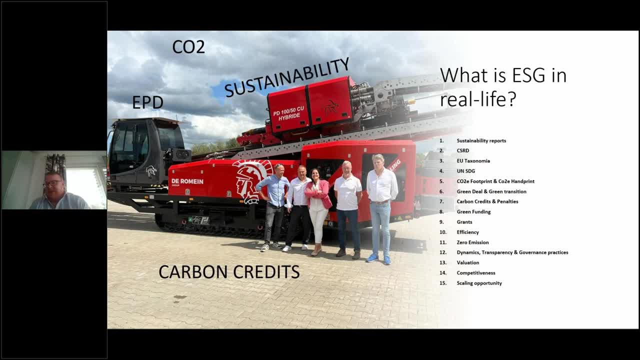 that 80- 90 off without esg. so it's so huge the impact. and top of that, everybody who is manufacturing is epd's environmental product declarations and they are local level, like every country can have a different population and can demand their own epds. so so that's one system actually to control the, the kind. 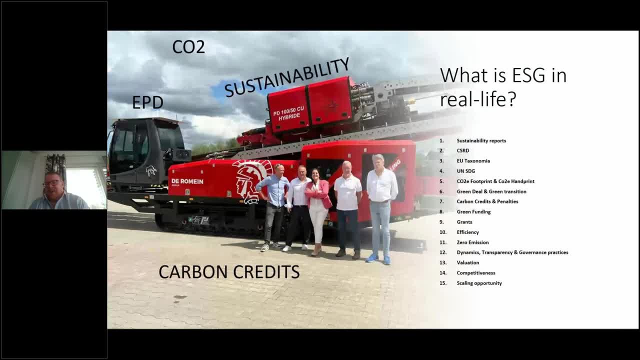 of import, export business, business inside europe and also globally. so this is how i understand the esg: like bit wider, and on top of it there is a lot of social impact, uh like more empowerment, less harassing impact when building, building and kind of opening roads and and. 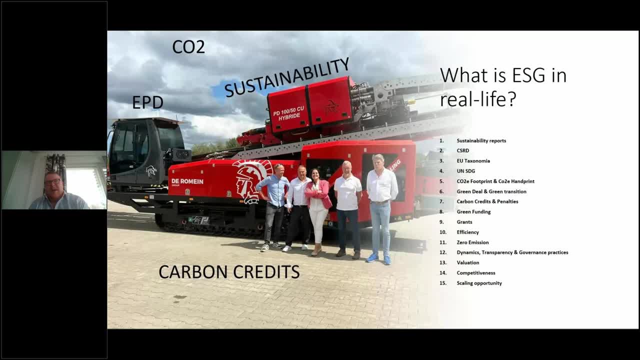 kind of making, making digging down tunnels and everything so much less impact to the people who are living around and when you do it faster, so it has always multiple times like a budget and co2 reduction and environmental people, people harassment much less. so every time is better. 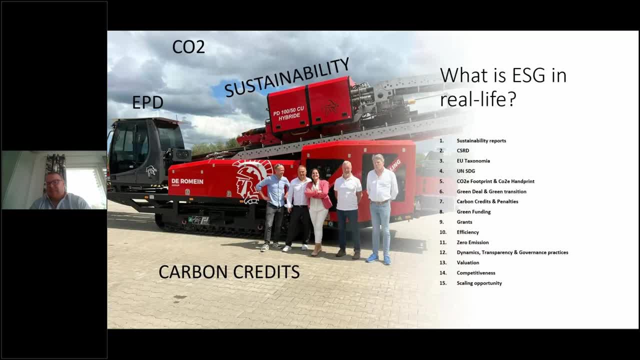 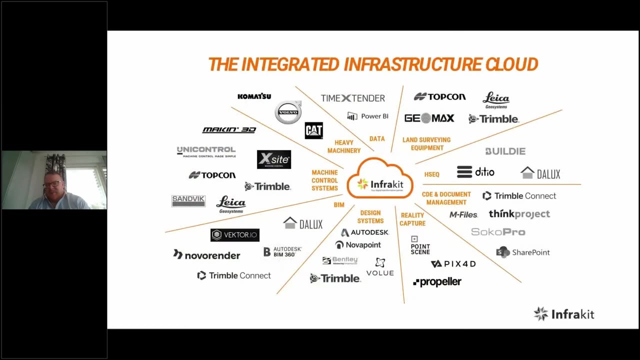 so this is how i see the esg, this is how i want to expand the thinking, if you can get the next slide. so then comes ecosystem neutral versus working with somebody. so how valuable is to be ecosystem neutral? so when, when i used to work for nokia, we were almost ecosystem neutral, but there was some. 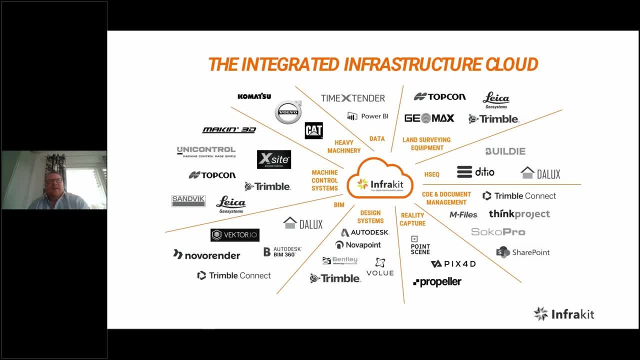 other ecosystems, like ericsson, for example. so from infracted point of view, we wanted to like increase our maturity of digitalization and all esg services for whole value chain. it means that we need to stay with everybody. you need to remain neutral, even they are very tempting offers coming. 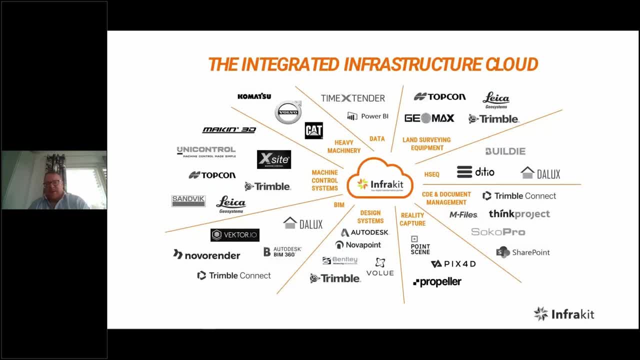 from a big players and they want, of course, maybe, maybe, to play a bit more with them. but if we can take all the data, so what is the outcome? in a whole value chain, there is all the planning design data data, all the building information, model data, machine control, which is in infrastructure. 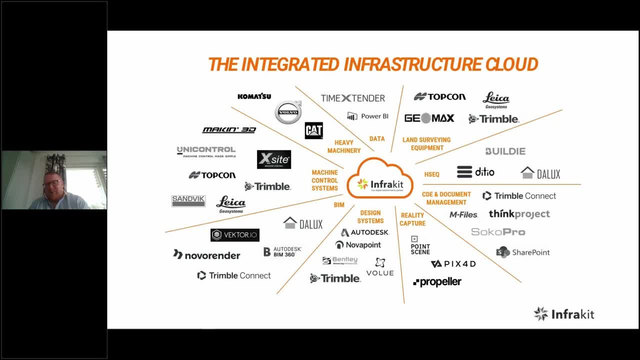 ultimate like two-way iq communication to giving the latest models, and then we have a lot of data we can show, you know in the dashboards: very accurate land surveying data, health safety, environment quality data, common data, environment data and then the like a thrones and any reality capture data. so together it's pretty much the same but it's a little bit different. 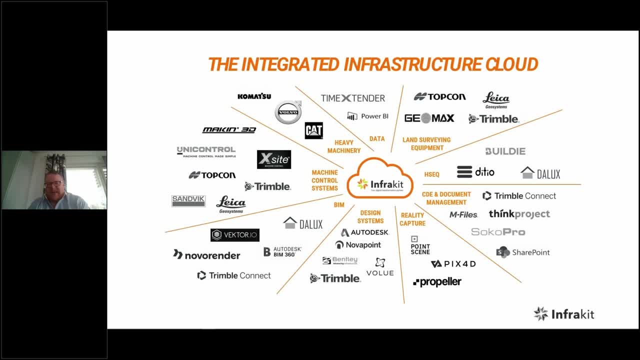 from what we have seen in the past. so we have a lot of data we can show you know in the dashboards. and then we have a lot of data we can show you know in the dashboards. much. no one can fool you because there is so much data that makes you more accurate. 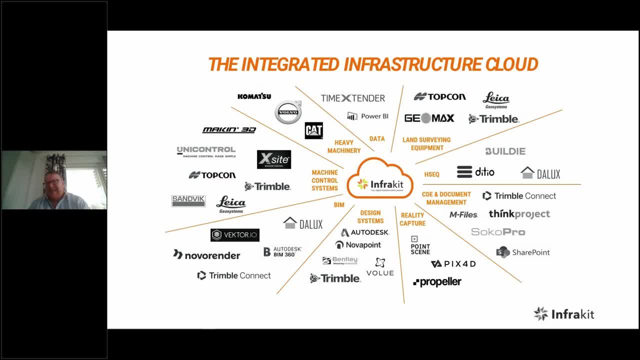 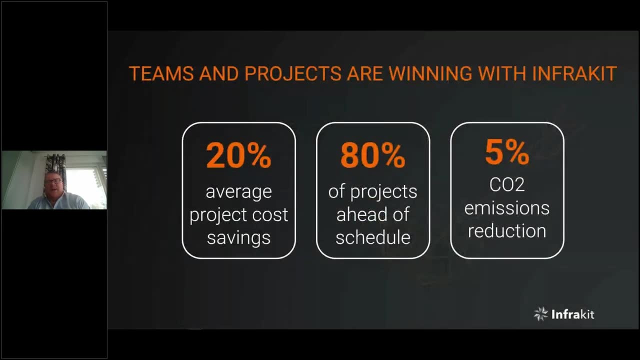 and now you have a single source of truth and you can share that single source of truth, and what might be the outcome when we just have this one and we don't need to do anything else. so if we get the next slide, please. so during the story, what happened to our customer? and they got acquired. so destia. 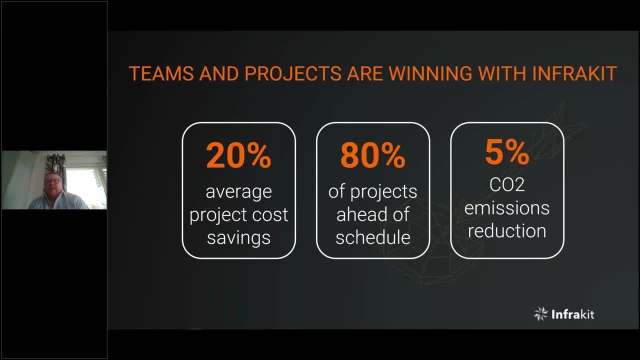 it used to be highest, before you forget, 145 million, and they got acquired by 500 million, so that's 355 million. valuation increased and it already happened two summers ago. and then regular infra project. it's about 20 percent as an average under the budget. then you just have this data like: 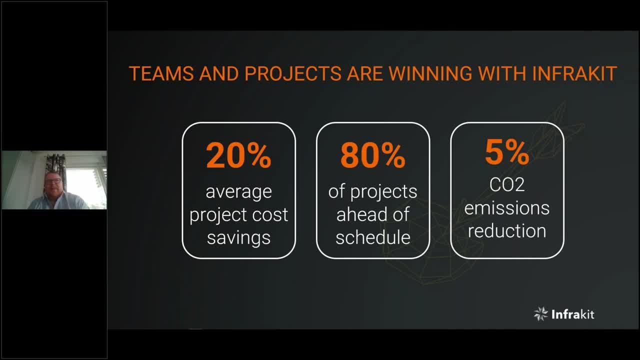 single source of truth, and not only on time delivery. our 150 last projects has been 80 ahead of schedule. so there are several high ways: railways, trams, airport expansions, harbors, there's even solar power plants and and the wind farms has been 80 percent ahead of schedule, and then minimum 5.6 percent reduced co2. but if 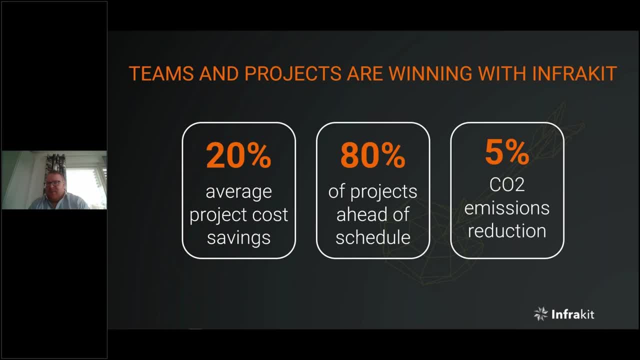 you take this under budget, so it's pretty much equal. get rid of waste, get rid of free doing and doing wrong things, so it's 20. impact also to co2 reduction. and if it's a 연pacto complication, call it, let's say 20. 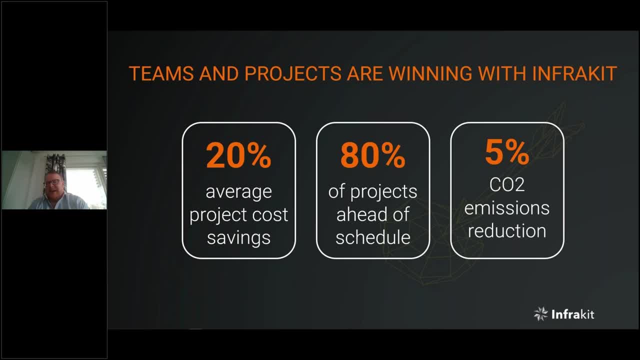 ready on time, or especially 80 ahead of schedule. so it has even bigger impact. so this verse 2 hasn't been calculated. it's just a very direct impact with efficiency. but this minimum 5.6. so it's quite significant when we know amounts of infra projects. 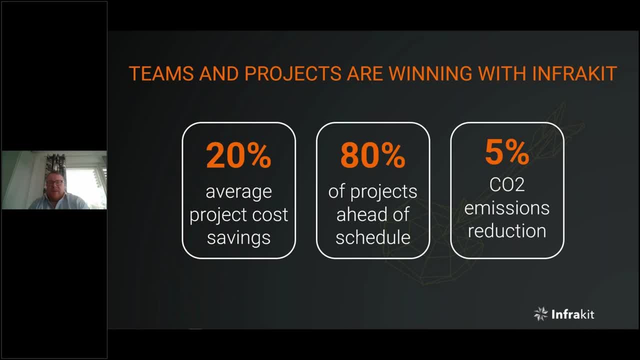 and uh. this is different in infra. if we need to go to real estate, like vertical building, the, the hammers and source don't have this iq. like machine control, water have applications for the for heavy trucks, so even that doesn't exist in the real estate. so in the construction site infrastructure is much better. but of course, even in infrastructure, 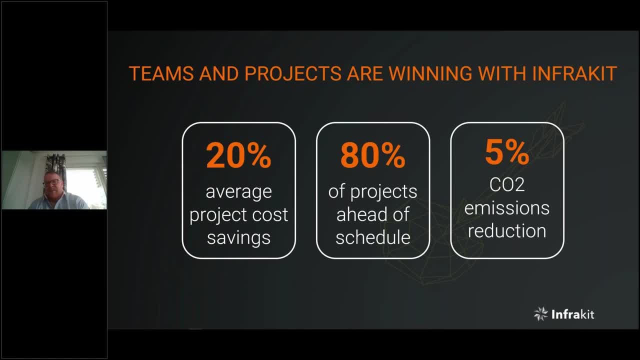 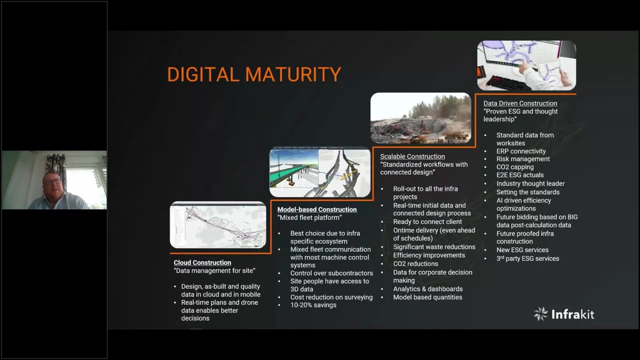 there is a lot to improve, for example, in handover to use and maintenance, but make a digital hand over instead of papers if we get the next slide, and that will be the most secret slide. so these are the maturity steps. then, uh, then talking with really, really smart people like you. 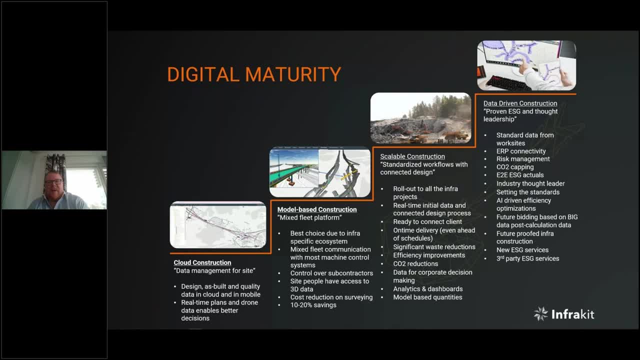 guys who know what's happening in esg, who has a lot of background, and i claim that, hey, we have been doing 6000 projects. i'm a third time traveling to every country and metropole in europe to understand esg maturities, and and then i say that this is for impact. we have been able to prove 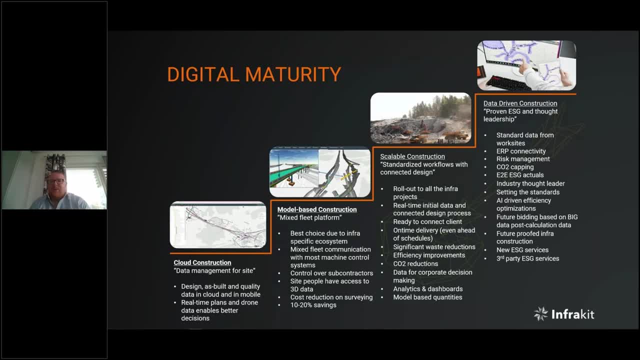 so, uh, customers have asking: okay, you know how to get there and you have done it with testia and many others. so what are the steps we need to do? and these are the secret steps: how to how to become number one in an industry? first one is digitalization. it needs two-way cloud and standardization. 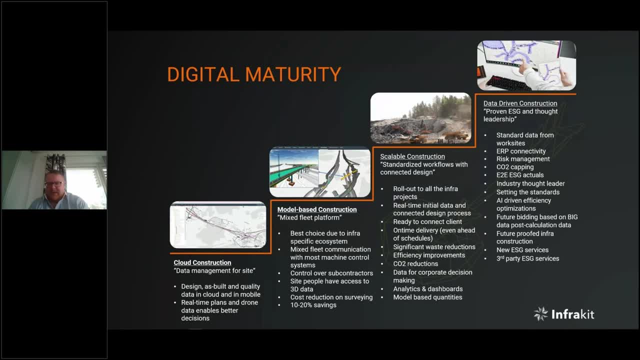 but you get the data in right format and you have all the data from all these integrations. what is relevant? second level is what you do with the data. it's like, uh, changing your process processes to model-based construction, and that's when you get minimum 10 and normally 20 percent impact. 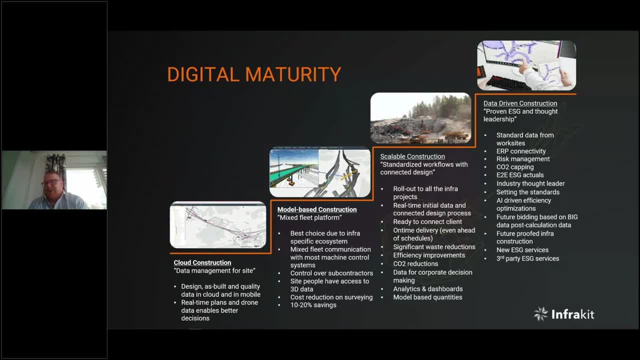 already into cost savings, so it's quite much when we talk about like originally 93 billion pounds hs2. so that impact would be in that word, like a nervous, and this we have been proven. i said thousands of times. so it's happening. just moving to model-based construction: little bit training. 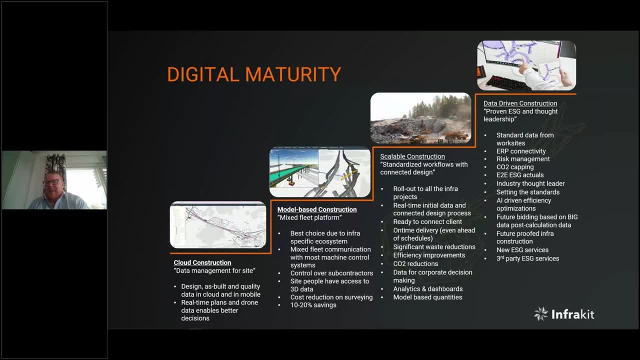 needed and we even have a customer success uh consultants to ensure it. the third level is you need to scale, but need to scale digitally, so that that is like taking this new way of working and write data into use in rolling it out to all the projects. that happens. 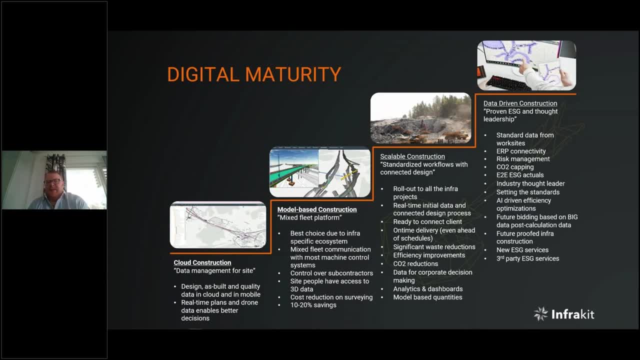 very efficiently when it's digital. if it's not digital, so it couldn't happen- but much bigger impact. you can multiply by project number the number of projects. this 20 impact already there, and then you go beyond because everybody is learning. it's like an iterative dance. uh, how we can make even bigger. 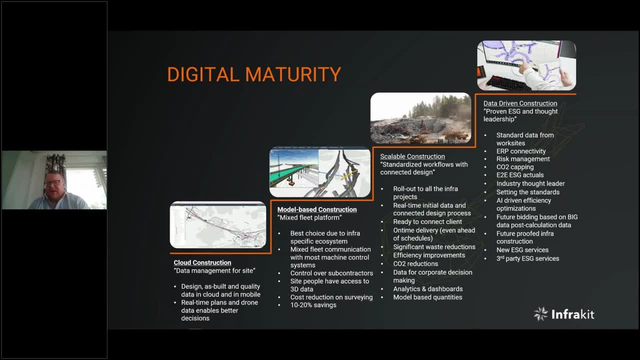 impact in a cost savings. efficiency demanding low carbon materials, uh, better energy sources like biofuel and electrification in the machines. so that's how we can get much bigger impact. at the same time, on the fourth level, when we already have all the data, we can set the thresholds. 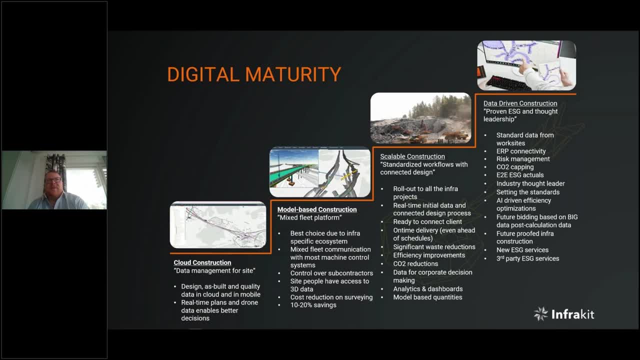 we can follow our thresholds real time, not afterwards in excel. if asking from a main contractors and subcontractors: what is, what are your esg, what are your co2s from the machines, and if that is done from a kind of buying fuel or something like that, so so i don't believe it. it should be what the machines are really using. 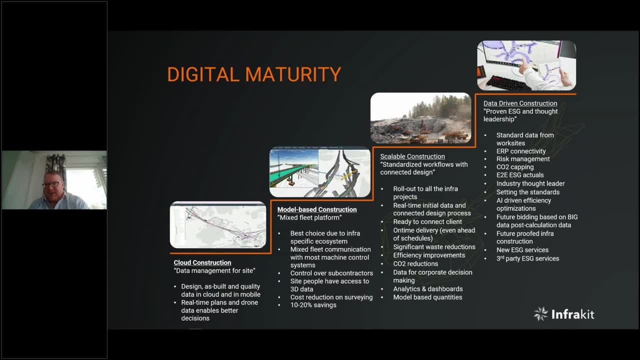 and uh, that gives the right facts and the kind of right values to compare, especially when we go to carbon credits, how much good we are doing and getting money back. so it must be always the actuals, and these actuals are on time, real time and uh, it's, it's much different. 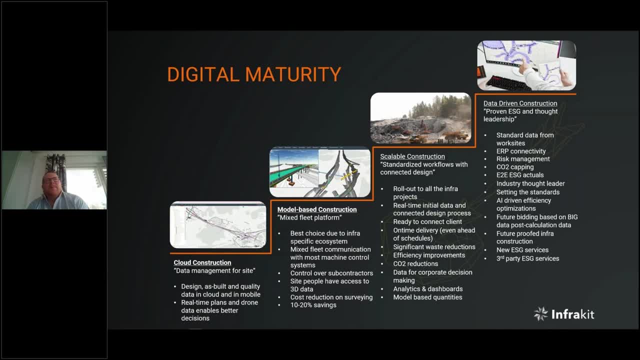 when doing it afterwards and you can also look like a, like a backtrack, like, okay, how much it was consuming what was with cost of of doing this part of the infra project. so you can learn and utilize even ai on top of that in the next bidding, like how to win the biddings and how to 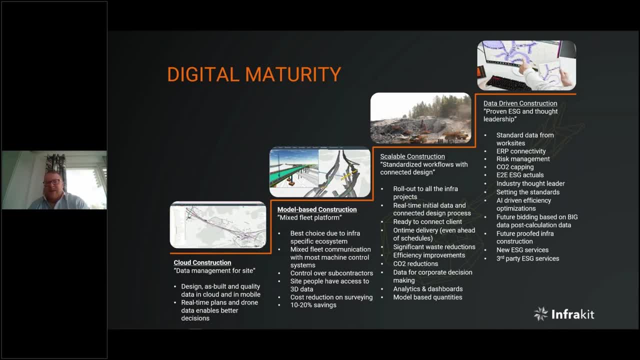 compare, as an owner, that which bidding is realistic and which are not, and then then always control the uh, the ultimate uh, co2s and the rest of the esg, esg criteria, because, uh, it will be in a dashboard every day. you can, you can look that and react on time, not afterwards. so that's called the secret. 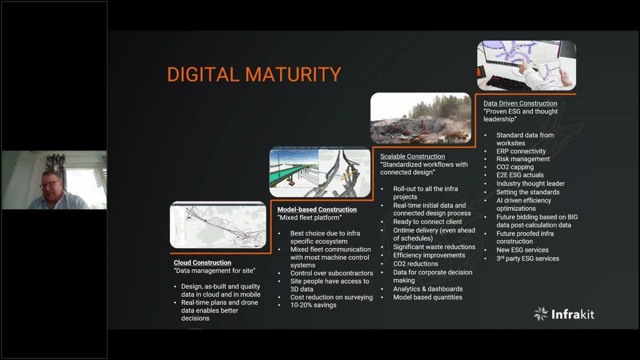 formula and uh, that's why the the ecosystem neutral platforms and, uh, that esg development has been really successful lately and we should be very valuable information. so that's from a presentation site today, thank you. uh, well, thank you very much. yako um a really good. 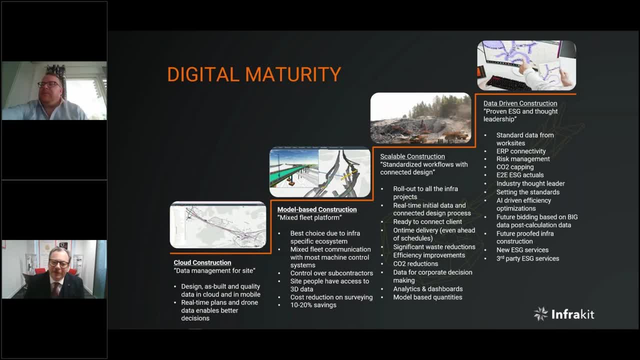 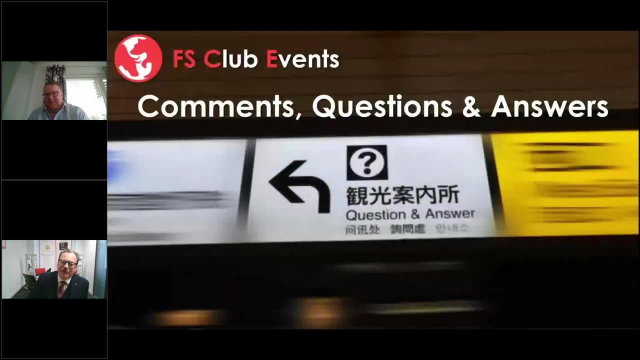 overview of um ways in which data-driven um systems uh can help i? i just wondered um you. obviously you've worked across the whole of the whole of the european network um. what variation do you see in the commitment of countries and the way in which esg is developing um in the 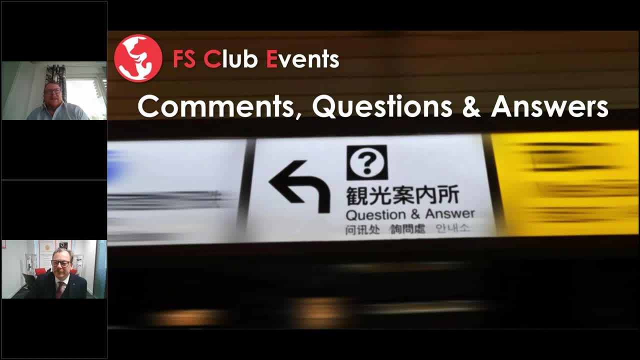 year. so that's, that's a really great question. i have been now two years, especially, uh, trying to understand the esg maturity in comparing the countries to each other and even within the value chain. so, uh, nordics are pretty good so so we have taken beam very seriously. but, uh, if we compare, we 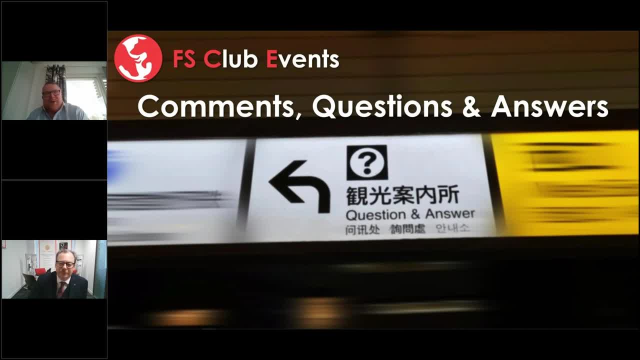 govern government part, so we london and uk is the highest because there's so much competence in the government part of the european government and the european government and the european government to demand but, um, how it turns to kind of, uh, how to say money and grants and actions, so that's. 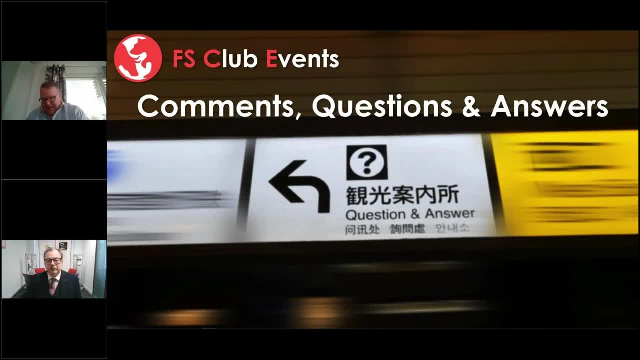 been better in in finland and in sweden and um in in germany. there is really much government support. we talk about uh a over 80 billion euros for for esg activities, but no one knows how to apply them. so it's it's like uh, when it doesn't deploy, the impact doesn't happen. and very lately the poland. 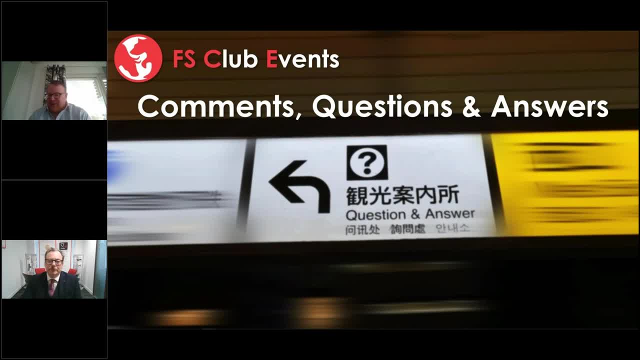 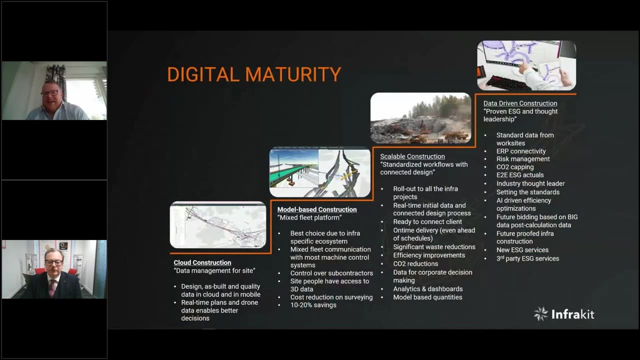 be rising. so one year ago poland used to be uh, against the esc and the government changed and they have really high quality ministers now in a climate and close to the european union. so they are climbing these steps right now the fastest. there is ideal location, really much money coming outside. 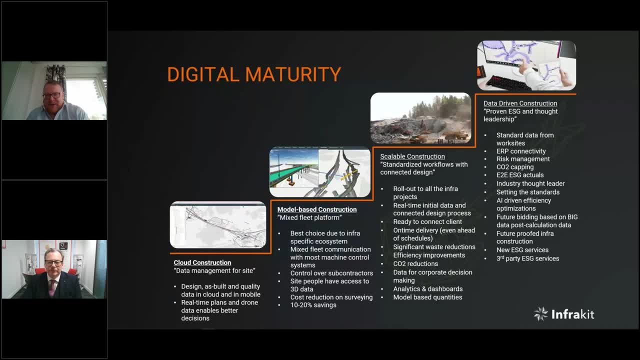 a lot of infra projects, so they want this impact and they want to do it like a sustainable way. so that's very positive surprise and and we have done one of the best projects in hungary and also in czech- czech. so, uh, these. i couldn't guess you would ask this two, three years ago. i would never guess that. 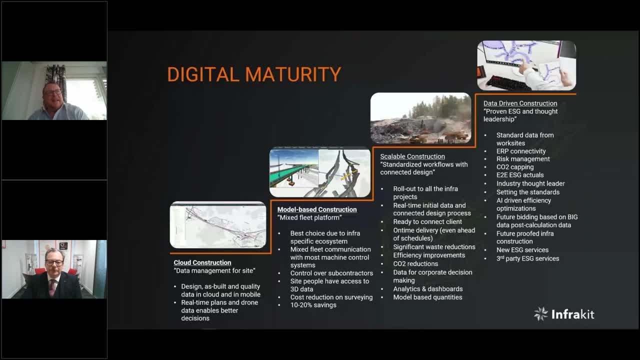 they are so high mature in in the market. and just yesterday, uh from, uh, from executive of business finland, i saw that finland was number one in esg maturity. so, uh, so that was also my finding. but then it goes in our value chain like government. 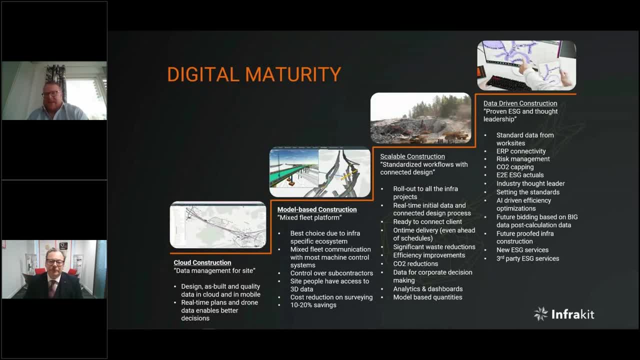 so it's really important role and owners like like that's, that's like a head of a snake and and uh, too much different but uh, but that's equalizing. now, always the highest matter has been architects like uh last 30 years playing with 3d- um, this little bit kidding like having good salaries. 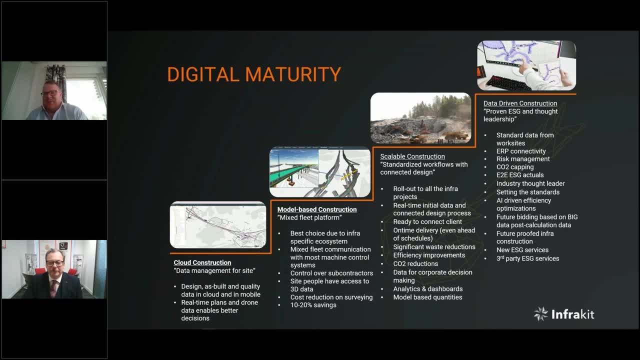 good life and also want to respect the next generation, so doing it sustainable way. so that's more normal for we, for the architects, but uh, then it when it goes to construction site. so before infrakit it was zero and now when infrakit, as a neutral platform, it has taken the infra. 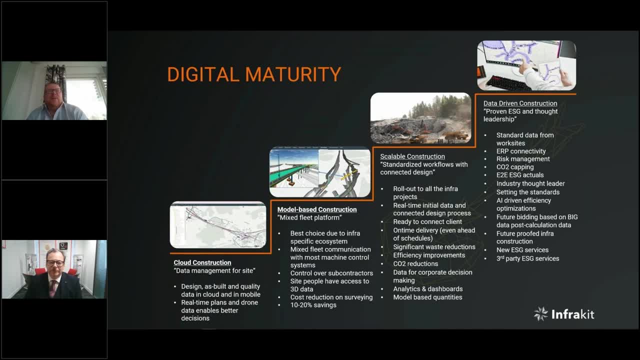 construction to very high maturity. but it has demand you should have machine control in our, in the devices. if that doesn't exist, so you don't get that accurate data and that accurate guidance. so for example, in finland machine control is 100 and and even top seven cities in finland has uh. 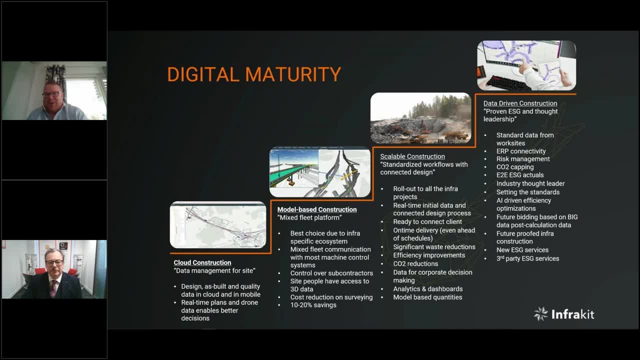 esg actual as a requirement that you can even work for the cities. so everybody in a value chain, also subcontractors, kind of knows how to do it. now that's also we need to collect this data. but then the biggest surprise: in use and maintenance, the maturity drops it. uh, there's like, let's say, three projects were hand over out of six. 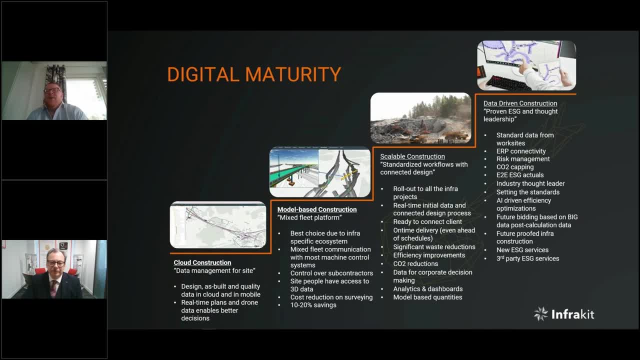 thousand which i know has happened digitally. it's still on a paper and it's outdated immediately. and one of the biggest, the biggest influence in very big end-to-end game of uh, for kind of a co2, for example, is use and maintenance, because, uh, it's very long time and- and comparing the couple of years- construction time. 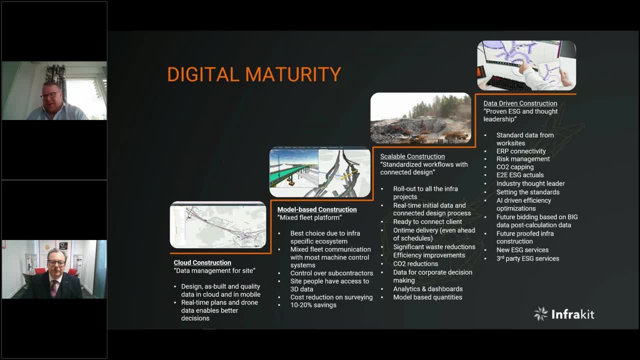 so, um this, this is something we can improve really much and we get really really good impact in a sustainability point of view and- and they are first ones- now making the real handovers and utilizing the latest information, and imagine when everything is documented really well, you know where the electricity, water, data lines are going, where the metro lines are going exactly. 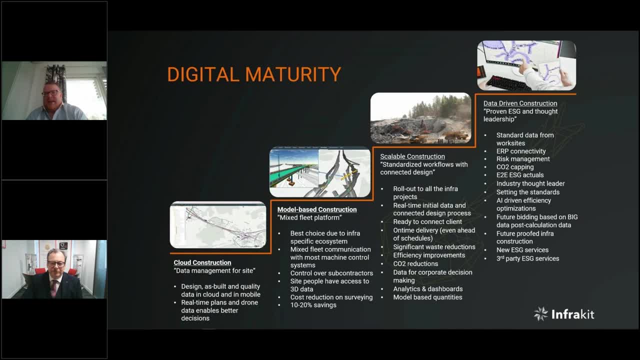 so nobody will make a mistake when everything is accurate. but nowadays one of the big problem is that they are definitely not accurate and and mistakes happen. and then it's a water pipeline in london broken by excavator, so there might be quite much water down down in the metro tunnels. 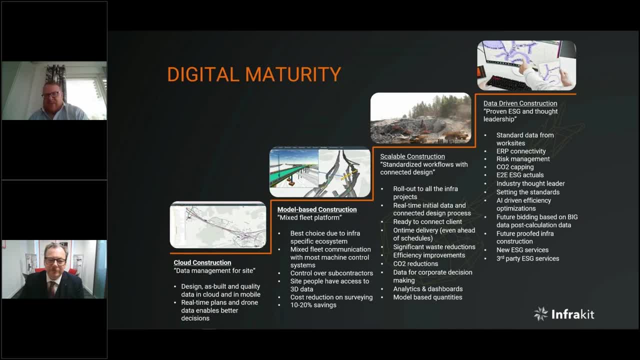 and so on. so, uh, so this accuracy in the next round will be automatically increasing the maturity of the whole value chain. and, uh, we, we have only first two cases in helsinki, there, the, the next infra project, has been like one third, because everything was correct in the beginning. everything was right. 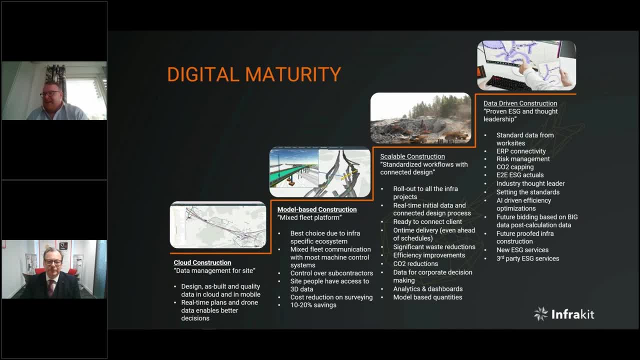 and if you compare real life without having having digital kind of a very good gps positioning, so they are not even close. so very interesting findings and personally very surprised about the differences. thank you very much. martin kember smith has asked about the co2 reductions. you're saying you're achieving five. 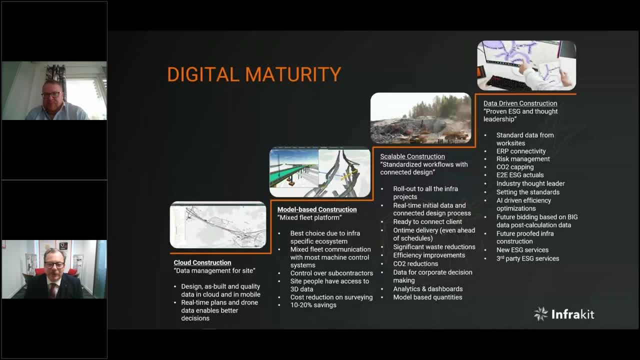 percent reductions? um, at the moment, is there potential to go much further, or is this, you know, hard to achieve? wow, so, uh. then we got a really good investment from a finnish climate fund and they demanded roadmap from us how to go to carbon zero in a whole infrastructure. and uh, there are a. 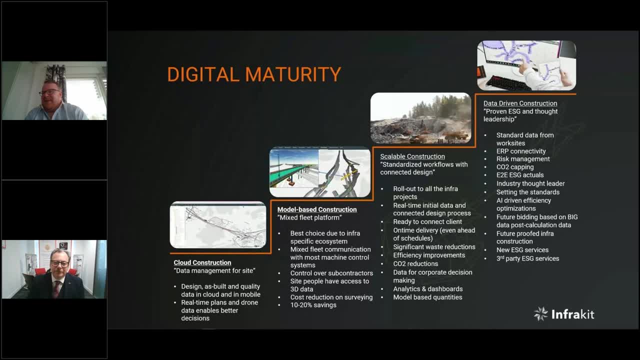 lot of cities who are nowadays claiming and and the kind of um, uh, how to say, committing to zero emission by 2030.. uh, i want to understand exactly, if it's now 5.6 percent as an average, how much we need to do every year, and it's not going to be easy, there's not. 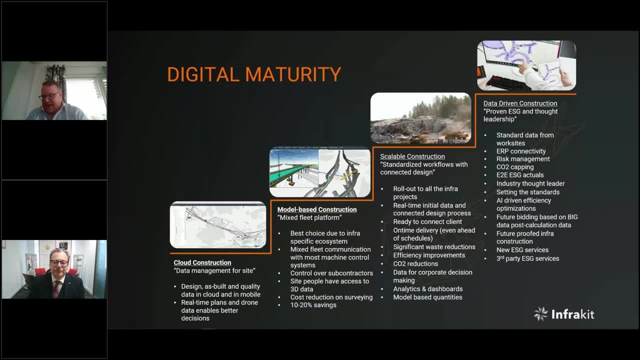 too many years to develop and deploy into into whole value chain that it will be 10 to 15 percent per year uh development needed to really reach 2030. but 2035 is uh is what office? it's. it's more doable, but how to do it? one part is efficiency. let's say 20. i have proven many times 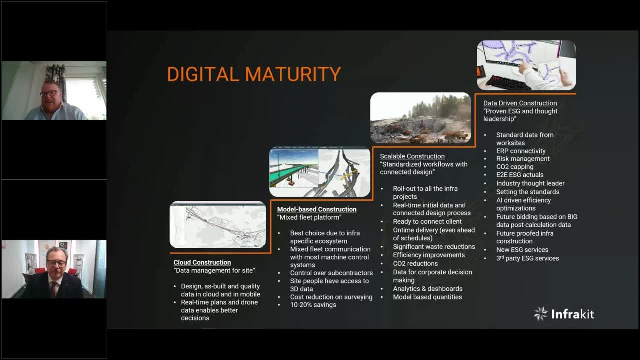 25 best cases. bit over 30, 35 with efficiency, but you cannot do more with efficiency. but when you demand materials like low carbon concrete or recyclable steel or green steel, that's like roughly 50 in end-to-end game input, like really huge. so demand materials, but make sure that these. 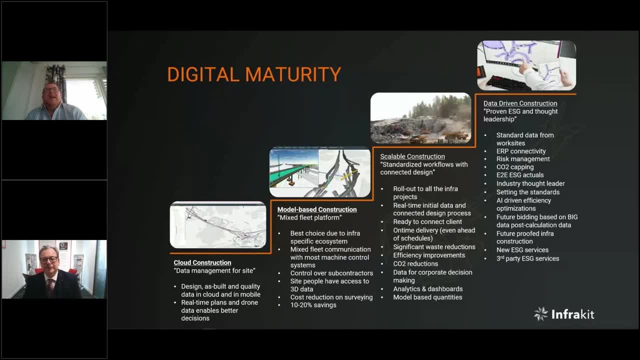 can deliver them on time and they are fitting to all the other criteria. then the last part is energy sources. we need electrification, as you saw, like a volvo cars did uh one month ago, the last turbo diesel car, and no, no more with traditional petrol cars are coming, so it's only 100 electric. 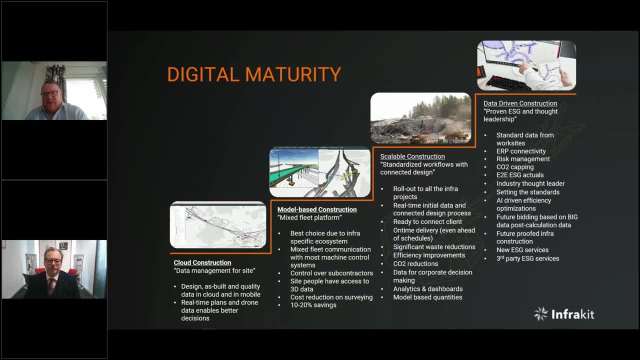 same happens in infrastructure and that has roughly about 30 percent end-to-end impact. so when we get all these, we can get carbon zero. but it means that all the in in a value chain has been deployed to this level and that's why 2030 i see very challenging. 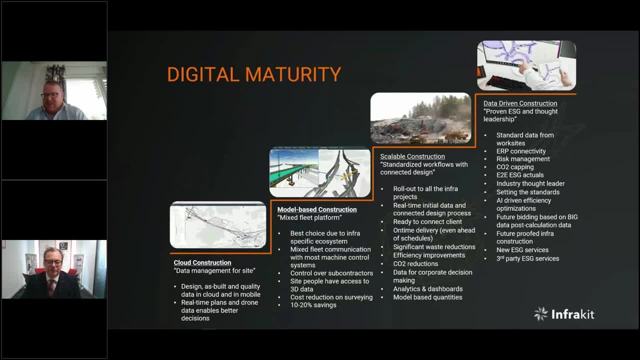 but, uh, all the good ones have started and i say, when you do sustainability, you get efficiency. you became number one and uh, it's also really good in the marketing after this under budget on time delivery or head of delivery stories. so that's why i see it very, very important. 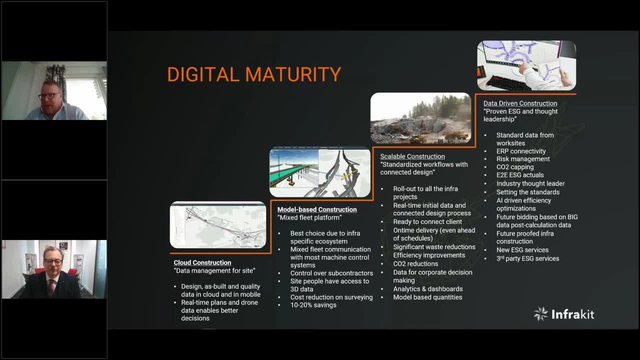 but hundred percent. on that task i also cooperate. i'm a chairman in a zero emission infra consortium, uh, especially where the person who was asking it is very welcome. welcome to this consortium, because that's where we do like. what are the concrete actions? how much you can demand nowadays, how about next year targets and so on, and we cooperate with owners. 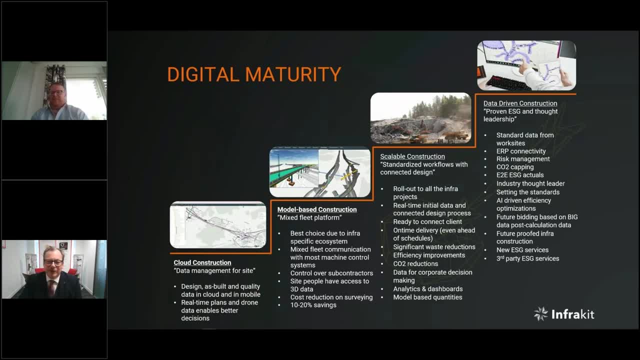 very close by- and i think shane drillion's asked a question which is in the same areas- really is asking whether the emission reductions that we're currently seeing um are they really coming from so far and are there real examples now of the mission reductions coming from adopting more? 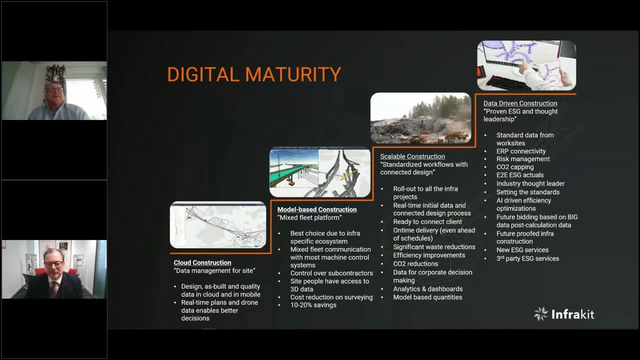 sustainable practices if there are no digital platform to prove it? i would say most likely not. if there is a really good digital platform to get the actuals all away from machines and machine movement, then they come from efficiency, of course, a little bit if you are really good. 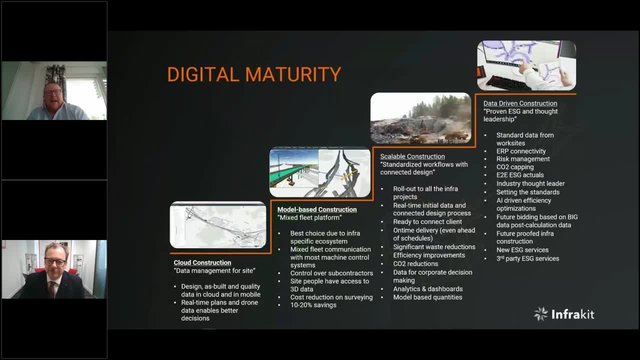 in planning in advance like uh, like minimizing the logistics movement and uh, optimizing everything, like uh, where you get your kind of uh, masses and uh and that. but in a, in a real life, uh, something get changed, other machines are waiting, wrong material is coming and redoing, so we need to get rid of that to get real efficiency impact. it's not even close to 20, if you. 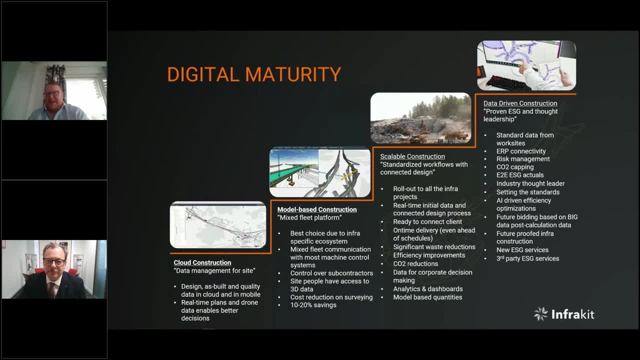 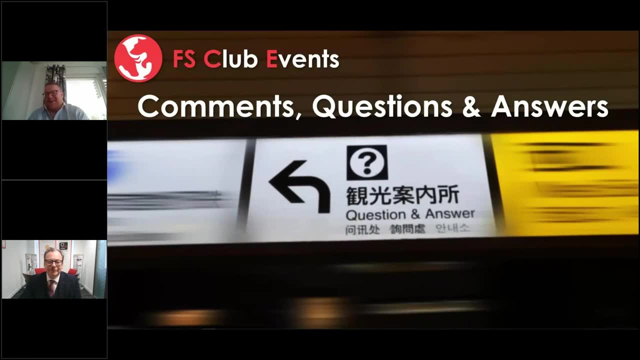 don't get the real on-site, like situational awareness and single source of truth, then it's doable. so i have seen that quite a few couple of hundred times. that's what we're doing right now and i i know what it is, but with the good help of planning so it gives better opportunity to get. 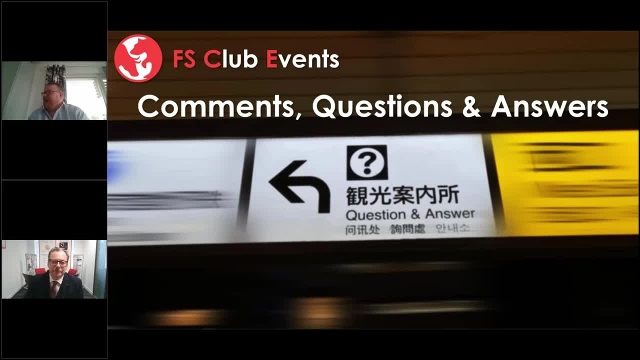 this 20 efficiency, which which is like, uh, it will be the new standard soon and it should be demanded, so it's a very right path. thank you very much. um. hugh purser, as online, has asked a question and he said: um, the discussion seems to relate mainly to new build for infrastructure. 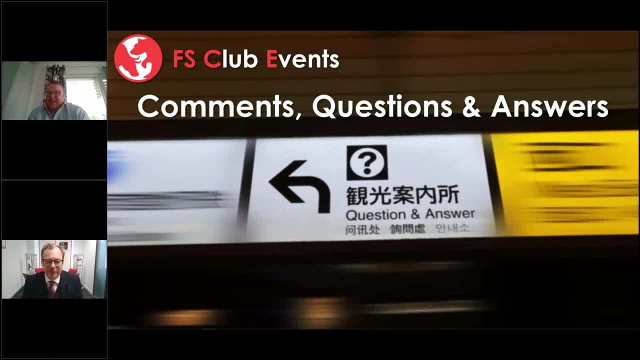 um, is there any development in analyzing improving current building and infrastructure stock? wow, okay, that's a tough one. so, uh, yes, it can be done. but uh, if you, if you go like a, there are bridges which are like buildings also. so if we can recycle the materials on site, so they paid. 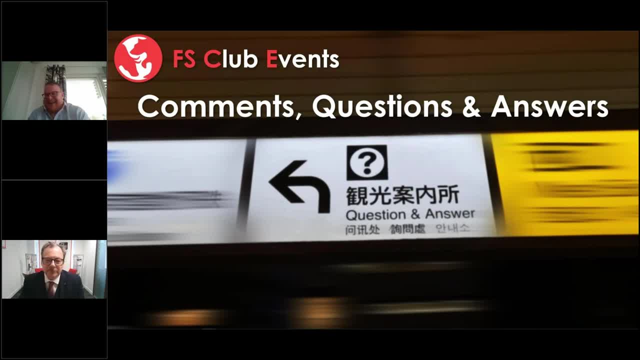 the penalty already in co2 emissions. and, uh, if you can do it on a way that it's not polluting and it's efficient and no logistics needed, so it's ultimately efficient. and now we have this material game, it's 50% and then to an import game, so that's marvelous. but if these materials doesn't exist, if they are, 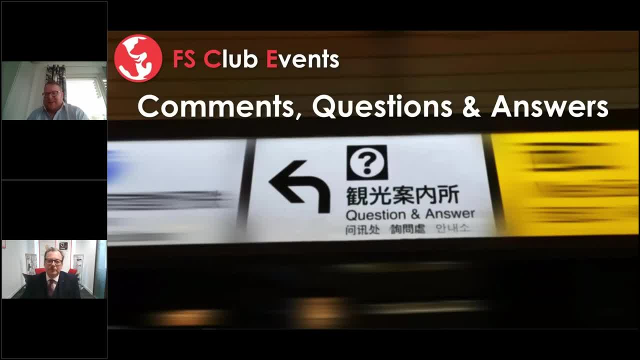 they are somehow like even poisonous or something. so you know which direction co2 emission goes in that case when we need to drive it very far away. so there are different kind of cases. there are. there's good and really bad cases. what, what i know? uh, from that angle, and of 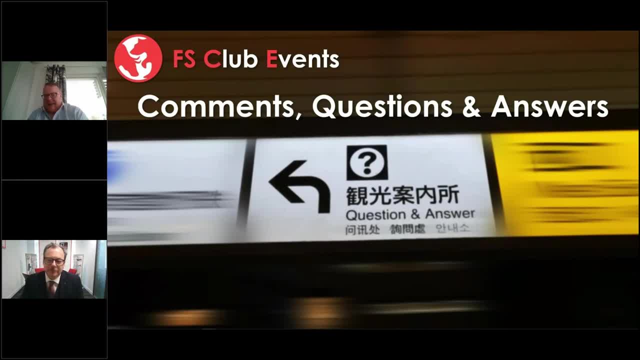 course, ways existing when we are redoing any, any infra in a big cities, when, knowing the long-term of this, there's, uh, several layers on top of it, so we need to be able to utilize everything we can and minimize this uh, but it's mandatory if it's, if it's bad material, so so we need to handle it. on the 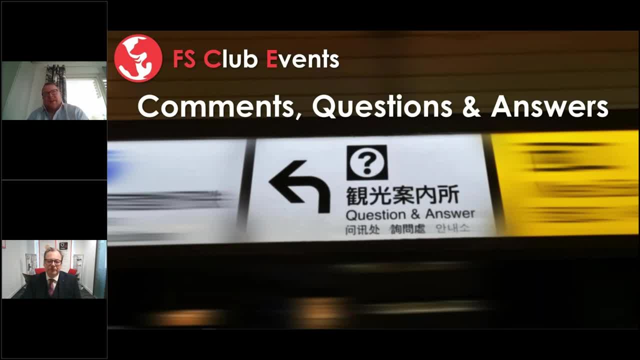 right way. but we also need to consider we water, like, like rivers and the waterways, so it's part of the esc, as equal as like a highway or or the, or the tunnel or the kind of more common infracases and and together these must be landed on a way that, uh, we can, we can kind of, uh, how to say, make 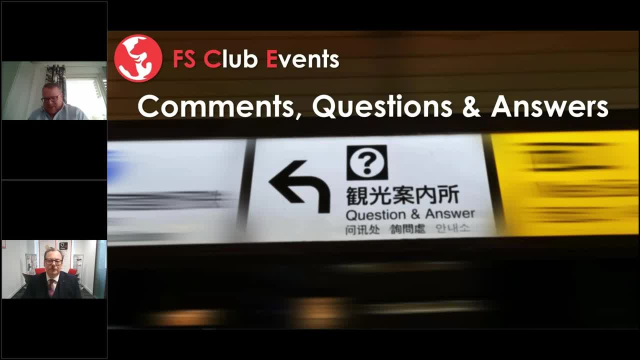 it more efficient, make it like, make it like a co2 reductions for, also for existing ones, because otherwise we don't change and we we cannot get the targets if we cannot touch the old kind of assets, assets also if it's only new ones, how to how to begin carbon zero? so it's impossible. 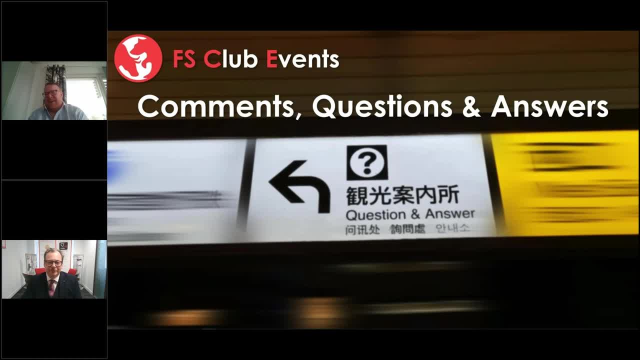 that's why it's very big part of it, of the game. and then, excellent question, very good thinking. thank you very much. um, i had a thought which is, uh, how transferable the learning that you've been through in infrastructure maybe to other sectors? um, and you know, where would, where would your imagination take you? 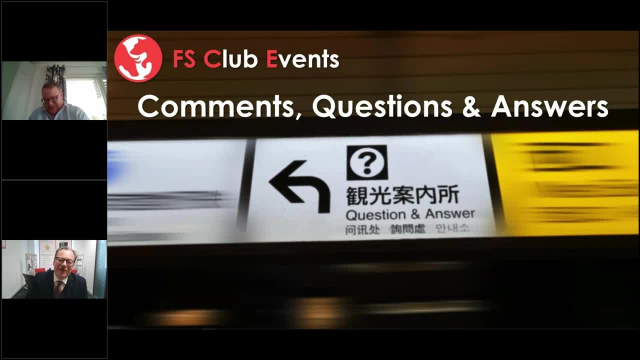 in terms of how ai and data-driven uh, esg might, might extend to other sectors. okay, wow, okay, one of my favorite thinking, so i would like to help rest of the real estate. i said there's so much asset assets there. the value chain is almost same from owners and the 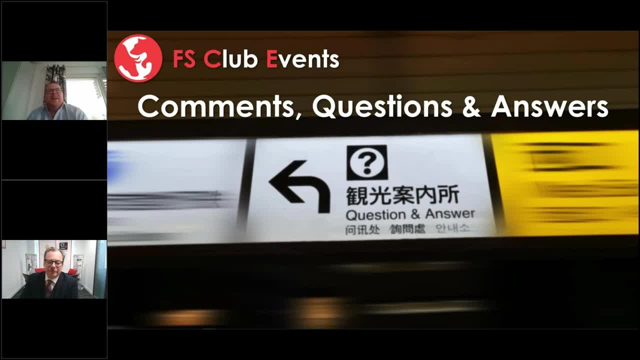 designers and they are main contractors. but on site the difference for the infra, comparing to like vertical uh buildings is- is very different because of his machine and machine control. so we matter to the difference is ultimate but the use and maintenance. actually the traditional construction has higher maturity, there is more. 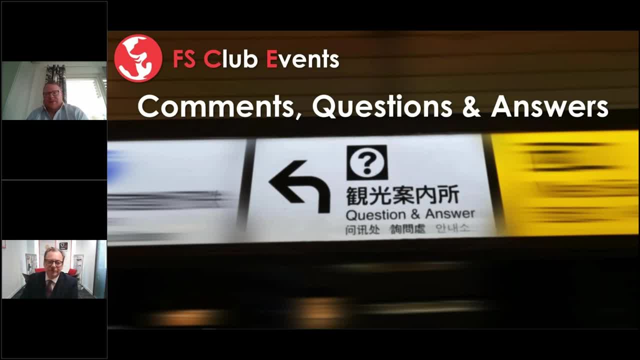 digital handovers. so thanks to demanding and doing a good job. so if we could utilize like best from above parts, that would be a very ideal case. then something very interesting: i was following 20 years uh with digital maturity of all different uh industries. 19 times the. the built environment was for lowest digital maturity. 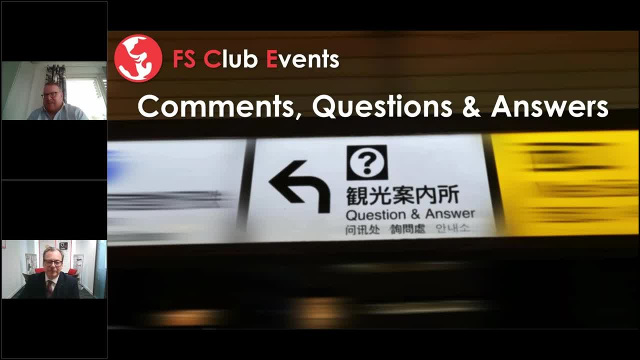 then i just learned that the infrastructure is 79 percent of greenhouse gases because energy pipelines are also moving there. so there's nothing bigger if it's 79 percent of kind of doing harm. so any good we do in infrastructure has bigger impact because multiplayer is so huge and and 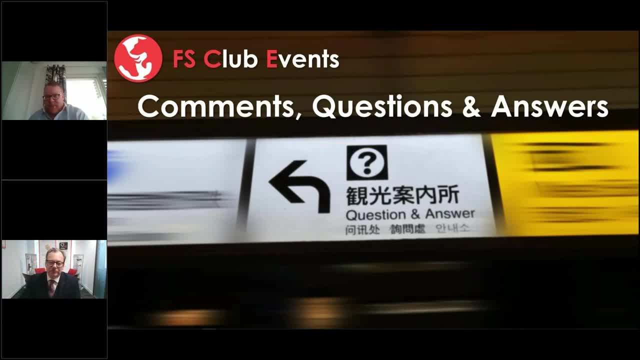 that is like bringing the infrastructure now top of the esg, like, wow, you are doing so much good. i said we used to be the last 19 out of 20 and and nobody was asking how you do digitalization. and now six cases. i have been keynote speaker. every time our impact has been the biggest. 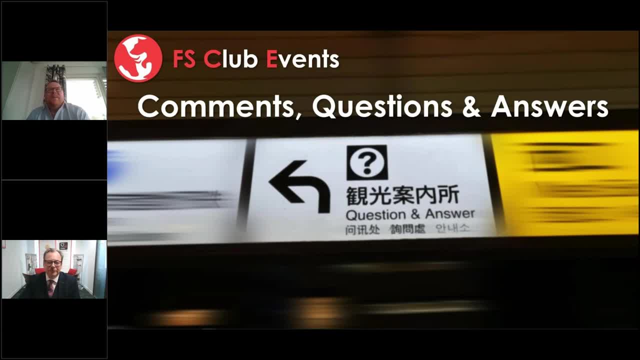 and and truly with 5.6 percent, like people you can. you can see sometimes 80 percent, 90, but even 100 percent reductions. so don't believe they are like in a silo, not in end to end. so it's not possible to do nowadays. five point six percent end to end. impact is so huge that uh. 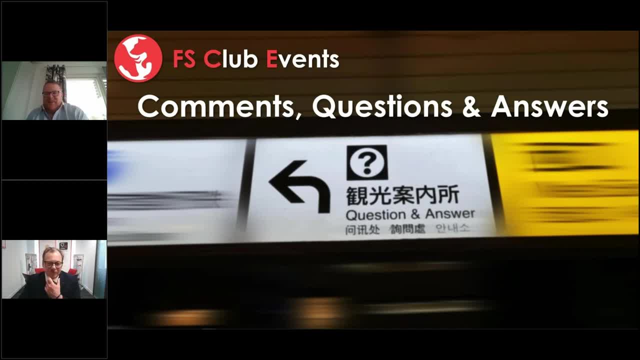 the, the best people, uh, in a climate fund? who? who compare these impacts between the industries? so they wanted to provide us more funding and enable bigger impact because of 5.6- and for me it was very small number when it was first time calculated and then everything was- 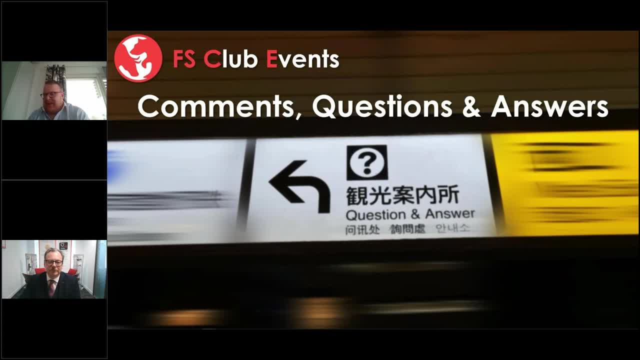 signed. they actually revealed that the impact with your 5.6 means every euro coming to your ecosystem neutral platform. every single euro is 30 kilos less co2 equivalent every single euro. so you are actually making the better world and that was like wow. 5.6 is so much because it's like a handprint- handprint impact that way. 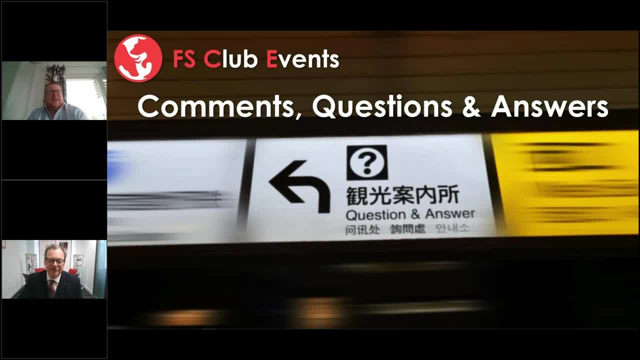 so definitely there's a lot to give to our industries and this time it's a really nice to be on top of wave. it's like again be like working for nokia back in the days. um, just turning to you mentioned, uh, your presentation the fact that funding is easier to get, um, when you have good esg. 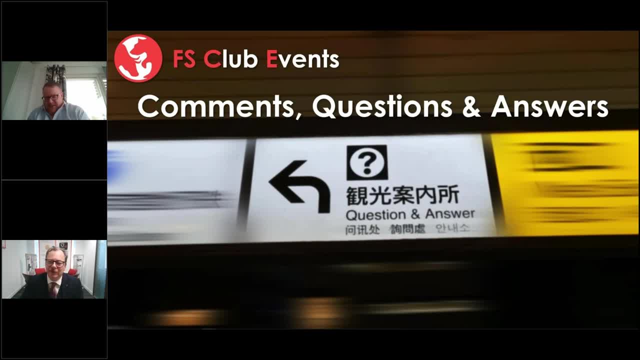 practices. could you comment a bit about that? and again, whether there's some differences between different markets. yeah, so this asset value is obvious. like, like in the comparison with uh, with the like with esg and without esg, the asset value is huge different. and there's so much green funds available and uh, they don't just give money, they need to prove so. 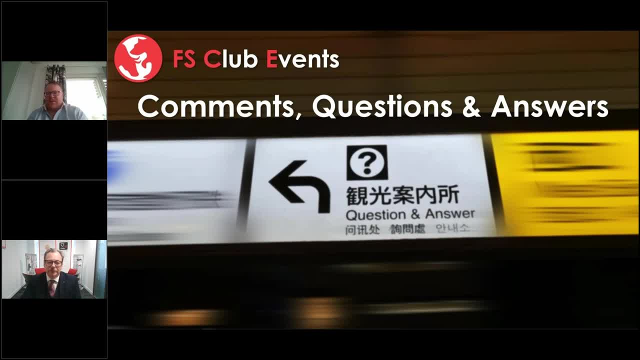 how to prove esg. you need data points, you need, you need to show like, like we are capable of doing it, and it's very difficult for the company. so if we need to go back into papers which are outdated or lost, so it's not possible to prove, it needs really much quality points in every part of the 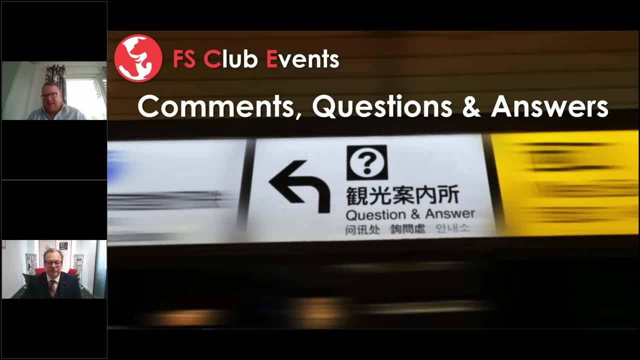 value chain. that owner has been demanding this kind of esg criteria showing the actuals, how well the efficiency, how well we materials, how well the energy sources has been fulfilling it. so that's really something. and then one more thing: part of the previous question is AI. 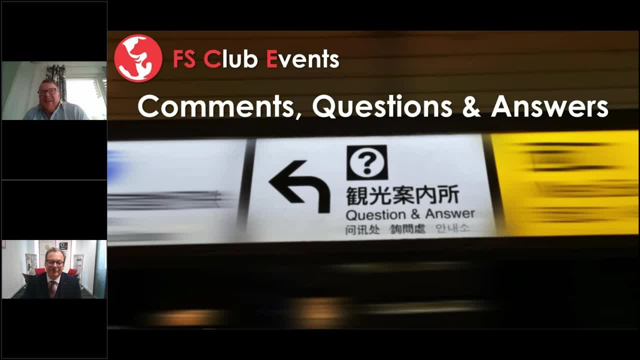 So I'm, and we are starting, so I'm heading the new opportunity to study the AI like impact to carbon zero in our industry. So now this is, of course, like we are estimating that it will be significant, but exactly how much? because AI loves data and now we have really. 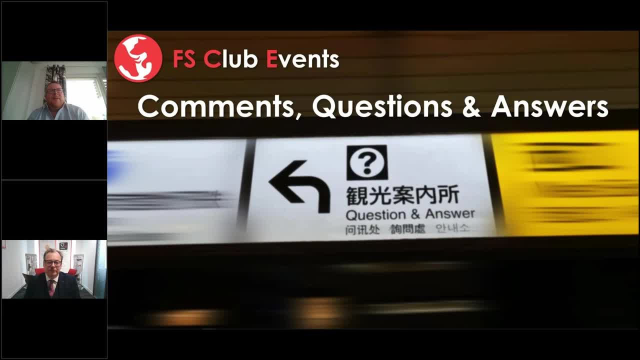 much data from different sources. So it will take away of mistake. It will. it will sell you about that. You kind of demand this because it's not doable. It will give the better kind of a impact of pricing, And it will. it will kind of give the owner like ultimate knowledge for sure. 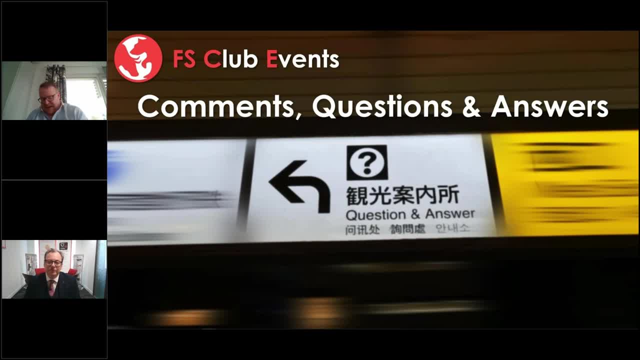 But what else it will do for everybody in a value chain, I would say really much. We will definitely see, but it will happen during, during this and next year's, not after 10 years. AI is already here And we are utilizing. 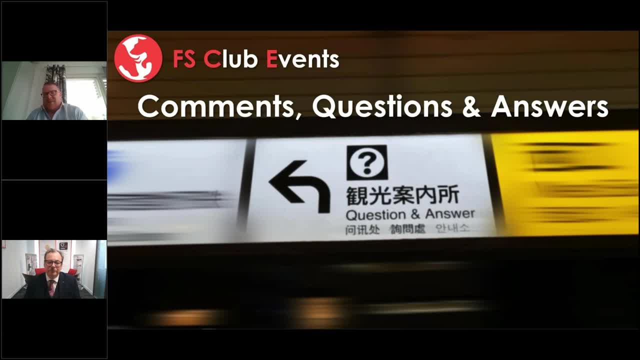 AI and more and more during next year for all the different kind of use cases, for internal optimization, for customer impact, for the owners, to to kind of make any infrastructure into faces for comparison and so on. And this is what we know now. If you ask this next year, my answer will be much better. 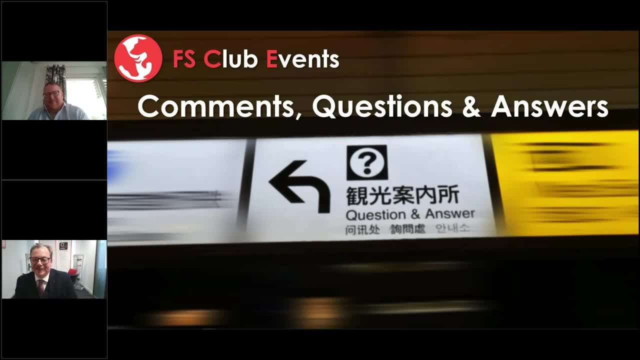 Thank you. Yes, it's a, certainly as a developing landscape. QPERS has come with a further question asking To what extent your projections take into account climate change, kind of either modest projections or the big projections. He's just noted The Economist this week when a big article on housing and climate change. 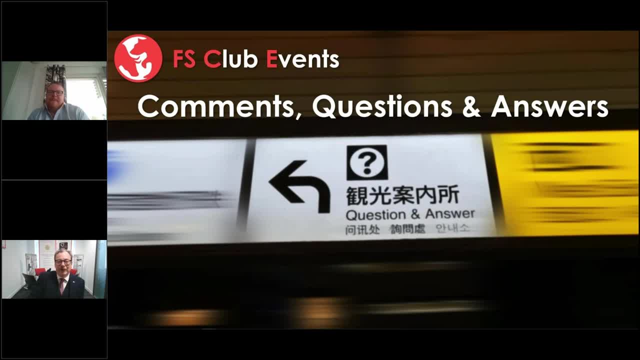 pointing to the potential of a massive valuation falls as climate change really hits home. Yeah, housing itself is 40%. I said infrastructure end to end is 79%, So I said there's nothing bigger. So if you only focus to energy, 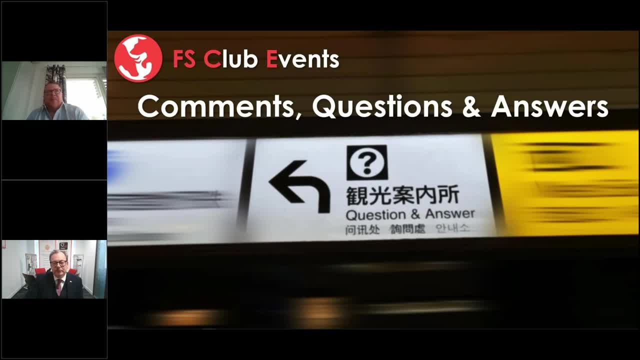 So if you only focus to energy sources like how to produce electricity, for example, so that's maximum 40%. So you need to move the energy. So it doesn't work if they are only in a plants and all the logistics- railways, harbors, airports, highways. 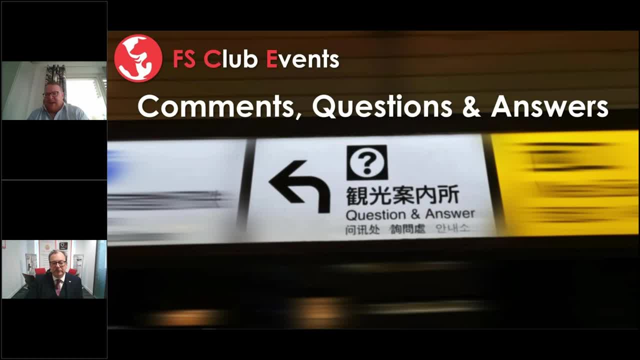 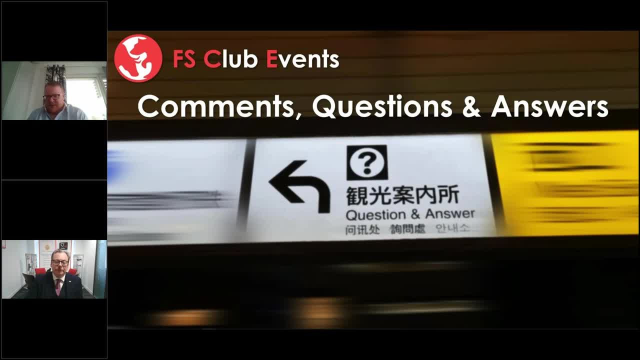 More sustainable. So it will need all these functionalities from ecosystem neutral platform, but also in the user maintenance space. So we need to take that user maintenance space more seriously and kind of continue there. There might be 30 to 100 years impact, significant impact, in that part. 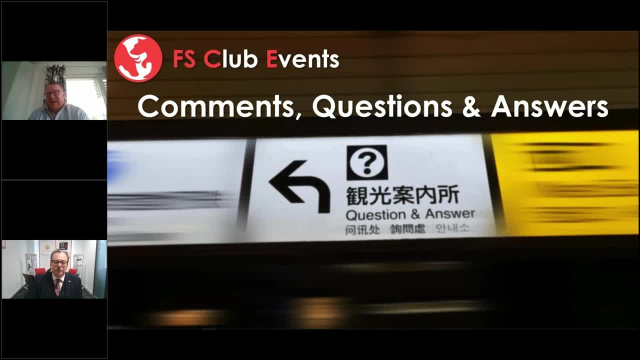 And I said I have seen three cases now doing it pretty much right And too many cases not not yet there. So one of the biggest improvement will happen there And Shane Trillian's come back to ask what emerging technologies do you believe are the most promising from an ESG perspective? 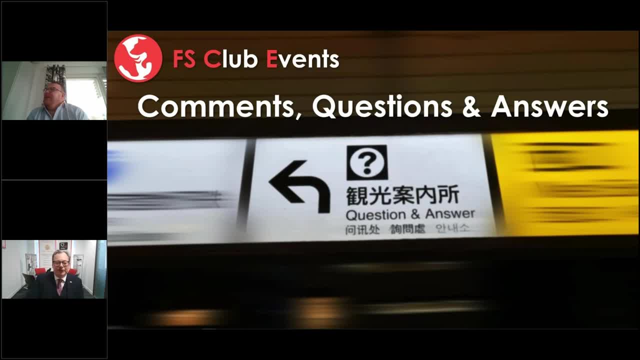 We talked about AI, but are there other? Yeah, AI is the next big, next biggest thing, for sure. I said there's so much data, So AI needs data, But it's also like there will be very many different kind of use cases and everything will be optimised, like telematics of the machines will be optimised. 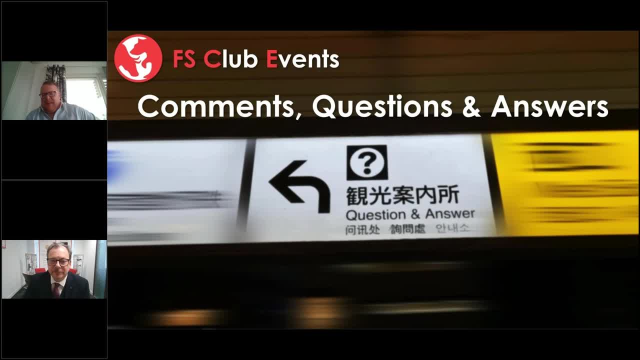 Material planning And movement will be more accurate. so, uh, it will be very easy to make bidding in in couple of years in an infrastructure, because you can compare to 10 000 projects that day and and uh, so, so all the gray areas will be disappearing. everybody knows the, the single source of truth. uh, kind of before. 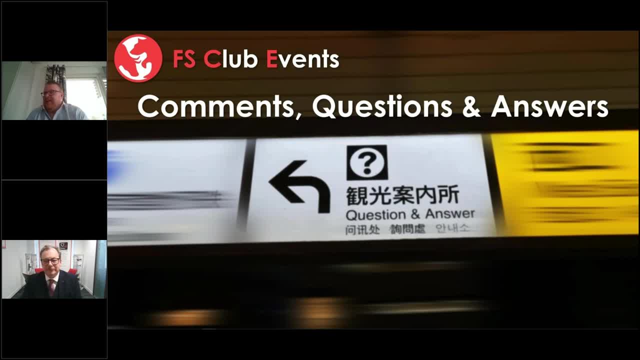 during and after, uh all the good guys will get uh kind of promotions. it's actually happening now in the cities in finland. so there's even one lady who has got two promotions during our cooperation already because it's so, so positive pr. so ai is very easy, easy kind of next thing happening and 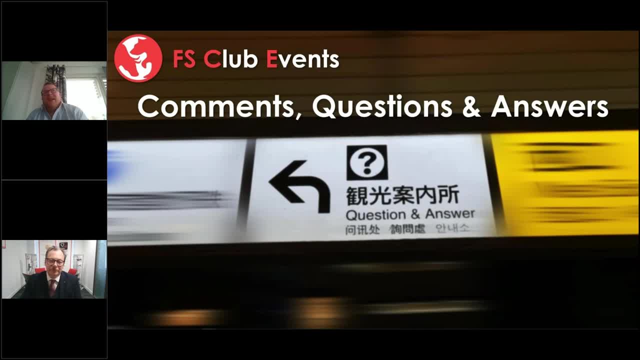 and we will see many formats, but uh. i would also say that that uh, everything like if you compare formula, once they have really good sensors, excavators has also but uh, but these sensors have been partly uh built in a factory and and the machine control have has been like after install it. so i will. i can say that within. 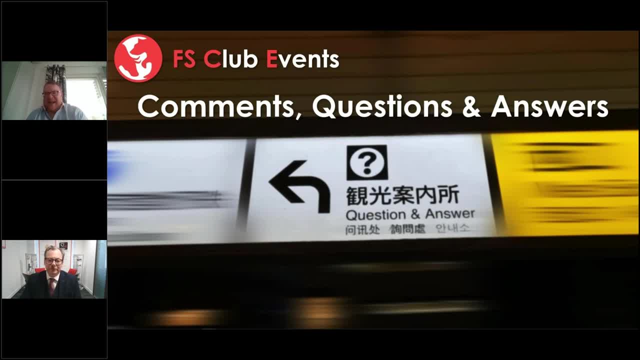 two, three years. they will be pre-installed in the factory, so it cannot be something afterwards and i thought. i thought that, uh, it's a small business so we talk about uh, all the top three companies in machine control are over billion euros revenue companies, so it's very serious. 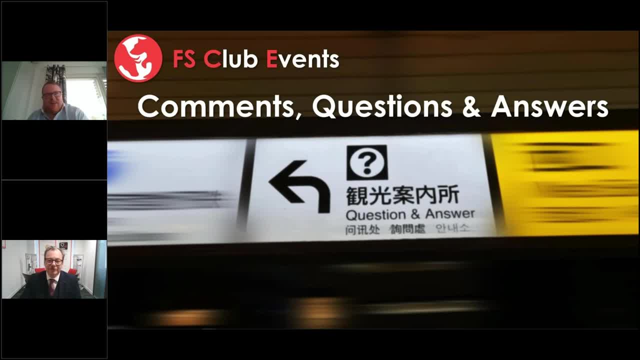 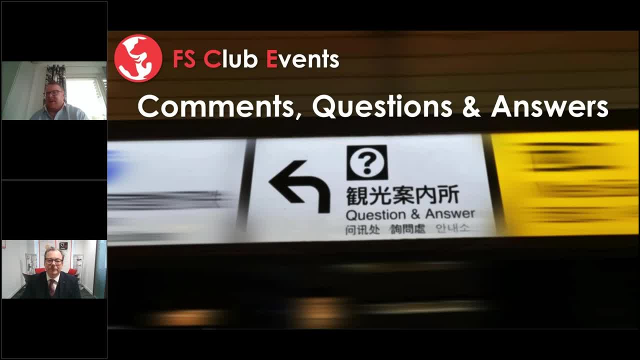 make it better, so it is possible that infrastructure will show an example of zero emission to all the other industries. it's very possible right now because it's very high material value chain. well, thank you very much. we we're coming to the end of the session, um, so just a. 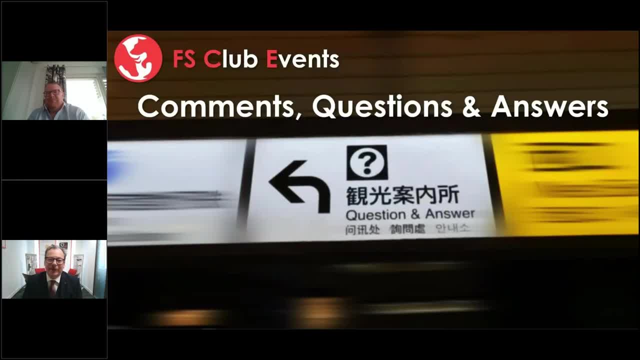 last question, i think for me, um, you mentioned the impact, for example, of the change of government in poland. um, you know, how far do you think is esg, development and climate change, adaptation and transition, uh, going to be driven really by government action? so, so the best governments? 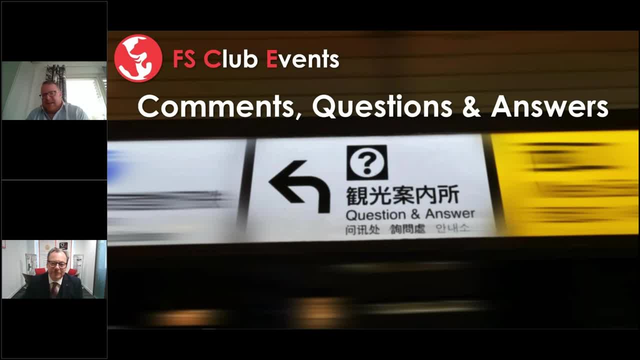 are demanding it, but when it gets deployed, uh, via cities, very well. so i said, seven out of seven top cities in finland has a hundred percent esg requirement. so you cannot get in if you cannot do the actual esgs. and all these projects have been ahead of schedule and the 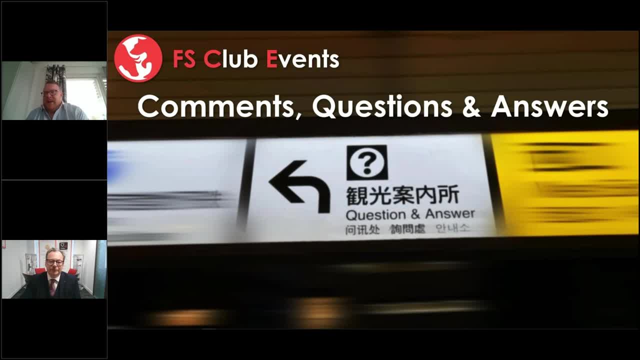 most important thing is that you have to have the highest quality and getting certifications- pream and the elite platinum- so it's like pushing enter when you have already all the quality points in a system in the right format. so we actually learned this from a huge nudic constructor who 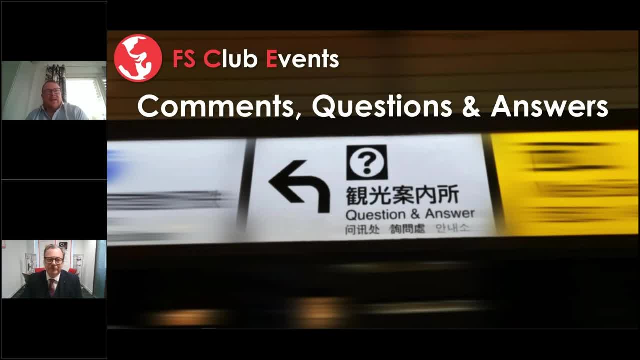 is working globally, especially also in uk, that, uh, they say thanks, guys, like it used to be very difficult to get certifications and now nowadays there's all the data in your platform so i just need to push enter. and it was not original use case, it was just a smart customer use case and 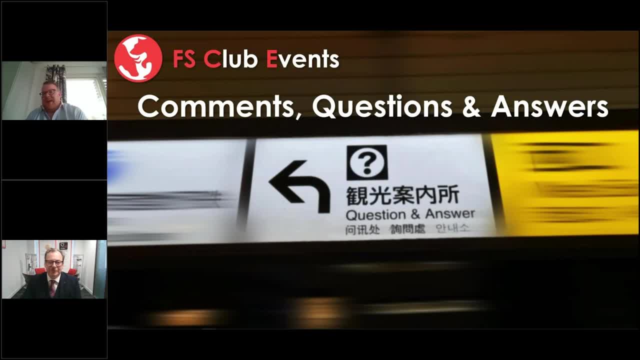 it was not original use case, it was just a smart customer use case and it was just a smart customer using it for for the right purpose. so i believe that this is all awareness which is now competitive advantage between of us. and uh, then, then it's 20 under budget. who wouldn't like it, especially as a 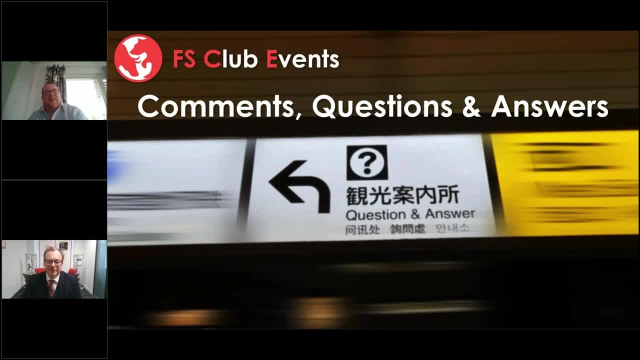 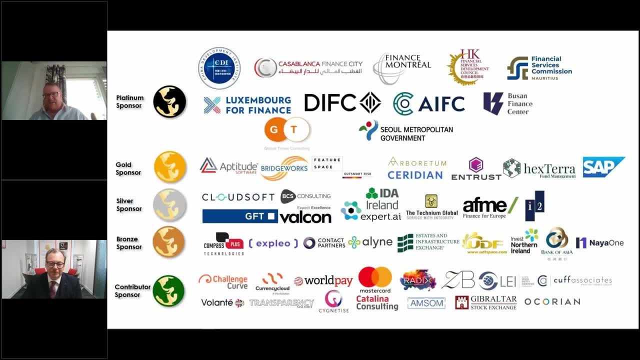 ceo. so so it's a really significant impact. so we need to do now this, what we have, and then together from 20 all the way to 50, 20, 30 and then to zero emission by 20- 35. so even we are neutral platform. 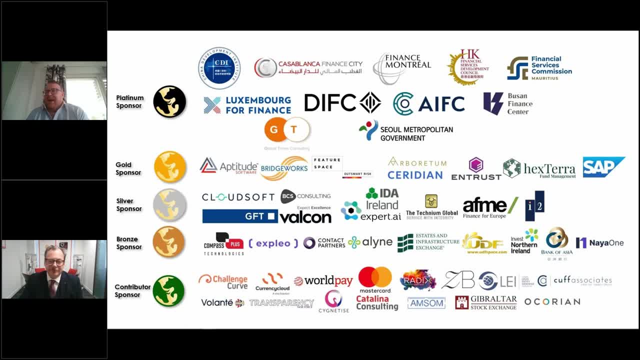 alone. we need owners, we need subcontractors, we need most likely some ai and technological providers and everybody in this value chain, but the outcome is going to be really good for us and really good for the next generation. well, thank you very much. um. a really good note, uh, to end on.